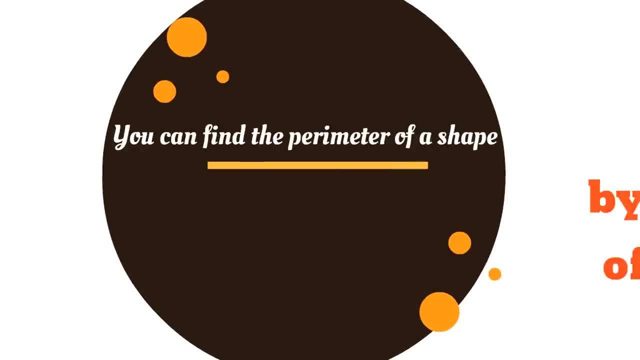 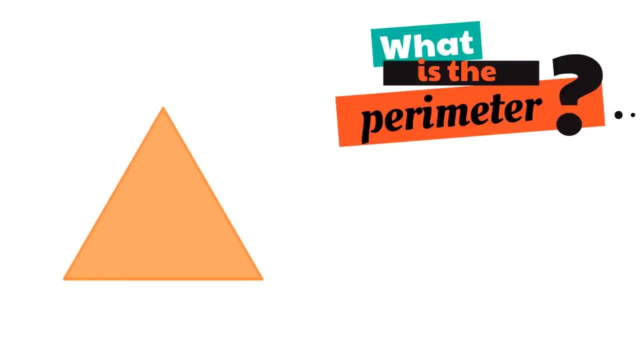 You can find the perimeter of a shape by adding all of the sides. That will tell you what the distance around the shape is Great. now let's practice finding the perimeter. Look at this track, Look at this triangle. What is the perimeter of this triangle? 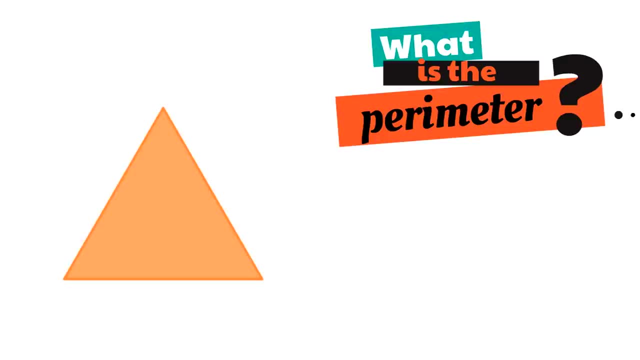 Okay, first we need to know how long all of the sides are. Then we can figure out the perimeter With this triangle. all three sides are the same length, So how long are they? Let's pretend we measured it and each side is 10 centimeters. 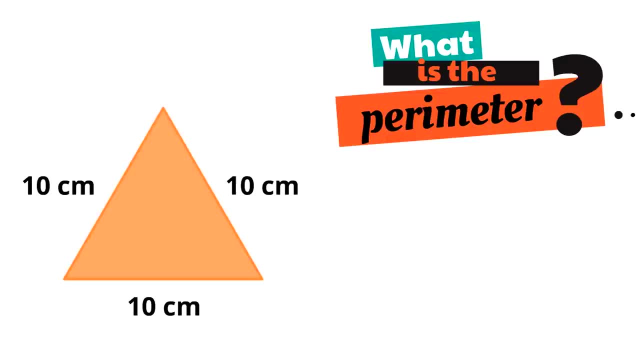 Now remember to find the perimeter of this triangle we need to know the distance around the whole shape, So we just add the sides together. What's 10 plus 10 plus 10? That's three tens. What does that equal? 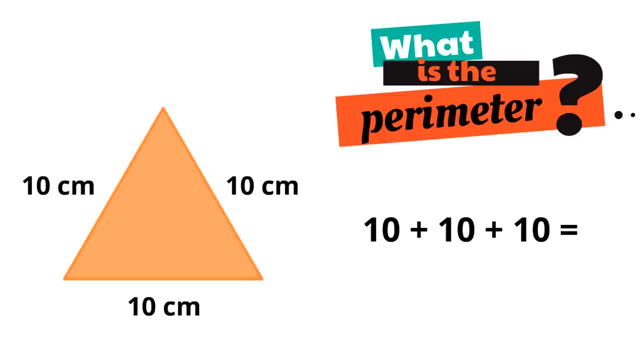 Yeah, 30.. Awesome, The perimeter of this triangle is 30 centimeters. Remember, CM is an abbreviation for centimeters: 30 centimeters, 30 centimeters is the perimeter of this triangle. Okay, let's try this one. 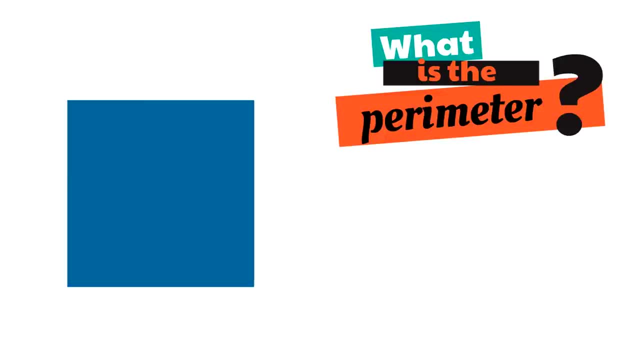 What is the perimeter of this square? First we need to know how long all the sides of the square are. Then we can figure out the perimeter of the square. Okay, so this is a square, It has four sides, And all four sides are the same size. 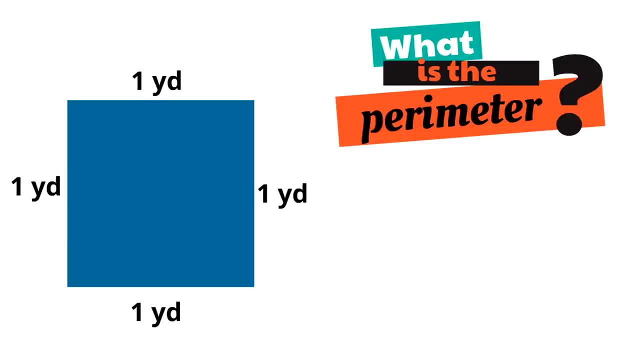 Let's pretend we measured it and each side is one yard. Remember, YD is an abbreviation for the distance of a yard. Each side is one yard. Remember, the perimeter is the distance around a shape, So we'll need to add all of these sides up. 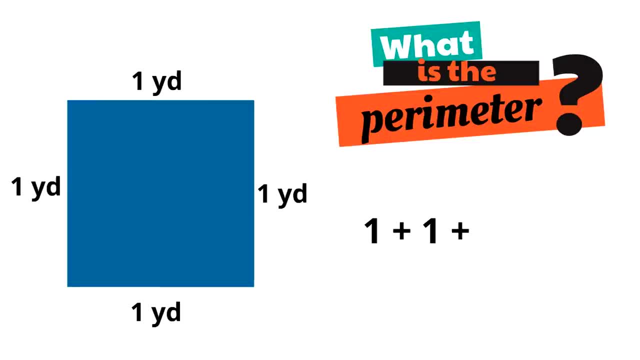 Okay, What's 1 plus 1 plus 1 plus 1?? Yeah, 4.. The perimeter of this square is 4 yards. The perimeter, remember, is the distance around a shape. If you were to go around this entire square, it would be 4 yards. 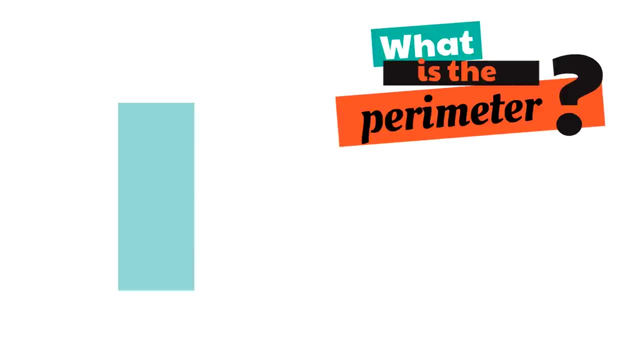 Okay, this is the final one. What is the perimeter of this rectangle? Well, first we need to know how long all the sides of the rectangle are, Then we can figure out the perimeter. Remember, a rectangle has four sides, And two of the sides are shorter than the other two sides. 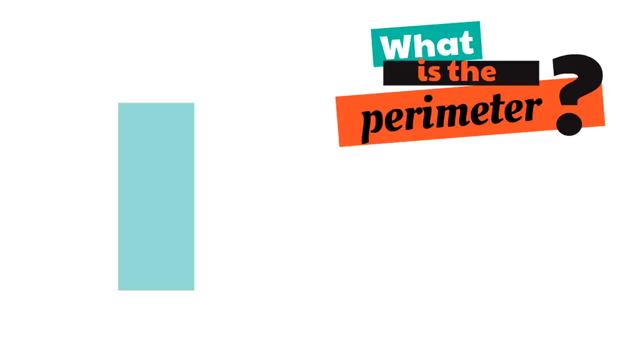 With this rectangle. let's pretend we measured it at one meter on the short side And 3 meters on the longer side. Okay, Remember, to get the perimeter we have to add all of the sides together, So we're going to be adding four numbers together again. 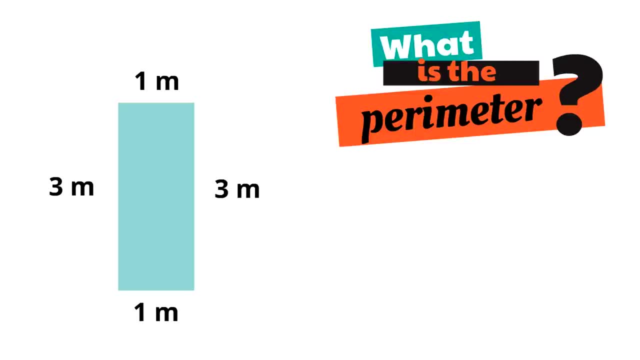 To make it easier, we're going to group the smaller numbers together and then put the larger numbers in our equation. What's 1 plus 1 plus 3 plus 3?? Those are all the sides. What's 1 plus 1 plus 3 plus 3?? 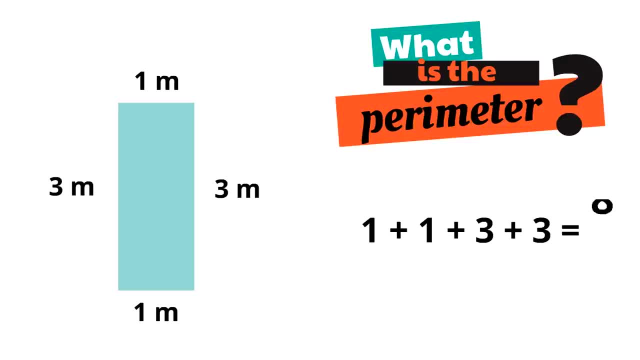 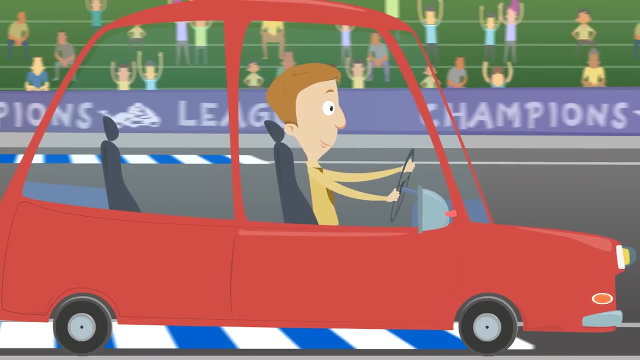 Yeah, 8!. That means the perimeter of this rectangle is 8 meters. Wow, we told you it was going to be fun. Oh, it's such a blast finding the perimeter. The perimeter is so much fun to find, It's like a game. 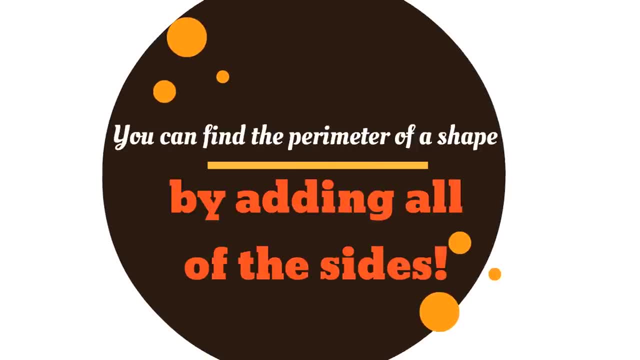 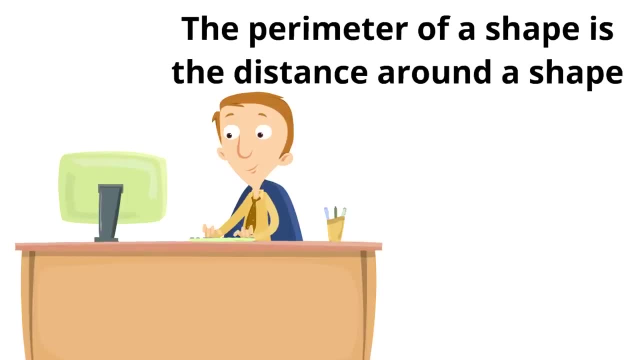 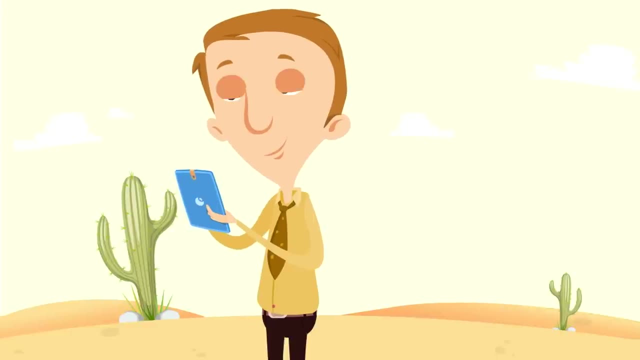 Remember, you can find the perimeter of a shape by adding all of the sides, And the perimeter of a shape is the distance around a shape. I'm so proud of you. I'm so proud of you. Now you know how to find the perimeter of something. 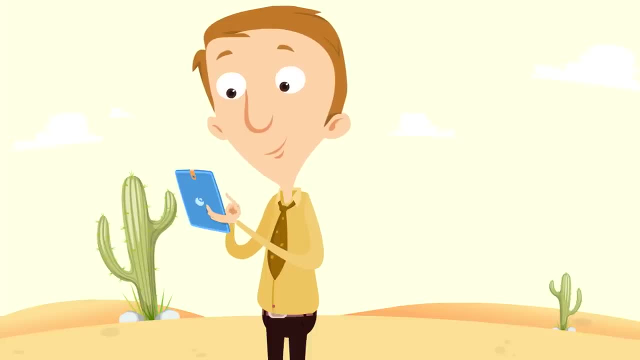 The perimeter is the distance around a shape. I can find the perimeter of this tablet right. All I would need to do is measure each side and add them together and I would find the perimeter. But right now I got to find an internet connection. 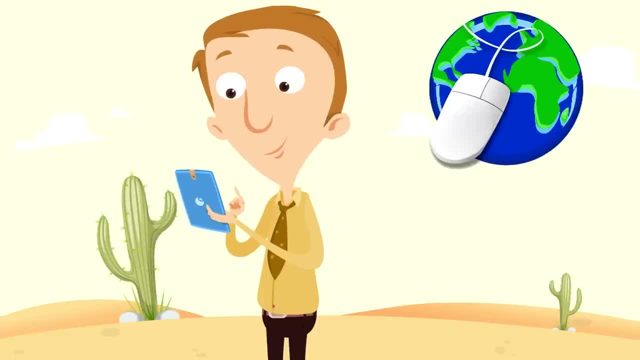 There's no Wi-Fi out here, There's no reason to be in the desert. I need water. This doesn't make any sense. Okay, so I'm going to go. You go ahead and find perimeter, Enjoy. The perimeter is the distance around a shape. 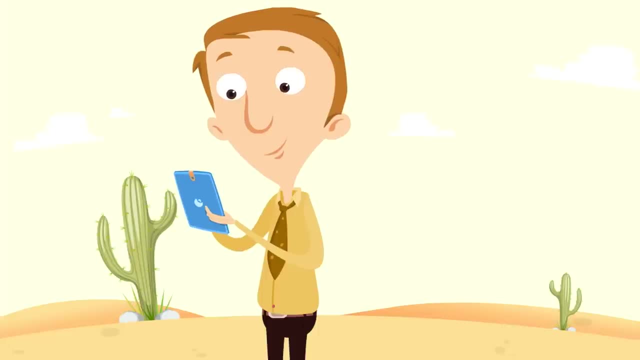 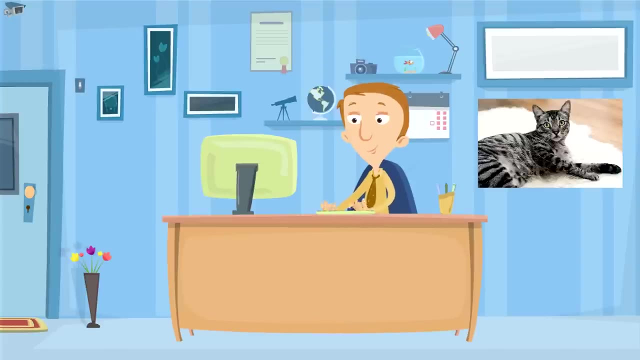 Go Have fun. Thanks for watching. We are so happy to have you with us. I mean, you are so awesome, You really are. Oh, you like my poster, Mr Whiskers' poster. you know, It's pretty cool, pretty cool, you know. 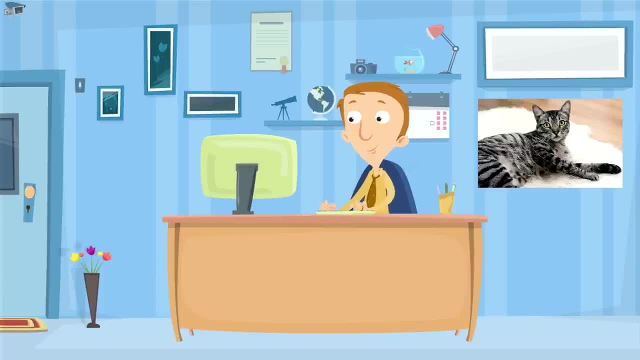 It's a pretty cool poster, Pretty cool cat too. I wonder what he would like to learn about next If he would learn from one of our videos. what would he like to learn next? Hmm, How about? Hmm, Let's learn about. 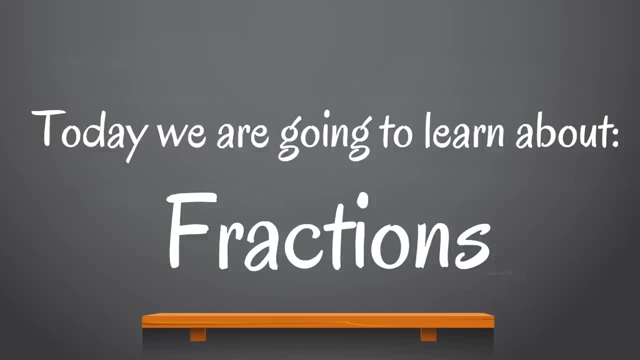 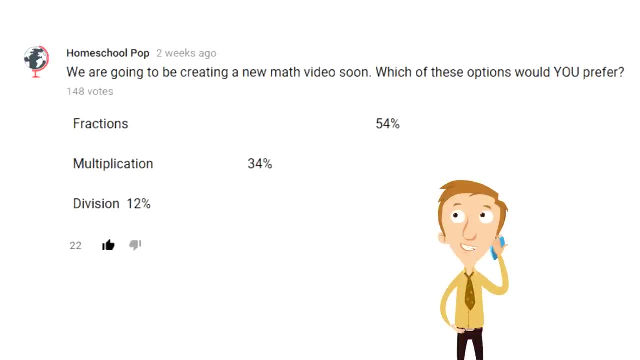 fractions. Fractions are so awesome and so much fun. Many of you think so too. A couple of weeks ago, we set up a poll on our channel and many of you voted for fractions as our next math video. That's really awesome. 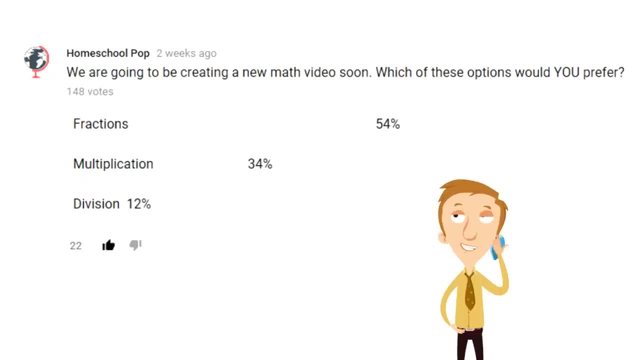 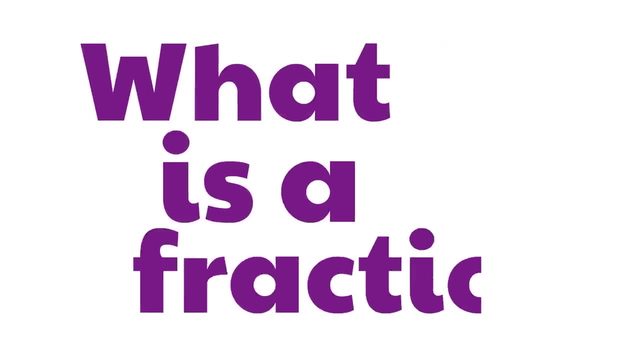 Thanks everyone for voting And don't worry, We'll make the other two videos too, Later on. But this is all about fractions, All right. Well, let's start here. What is a fraction? When we say the word fraction? 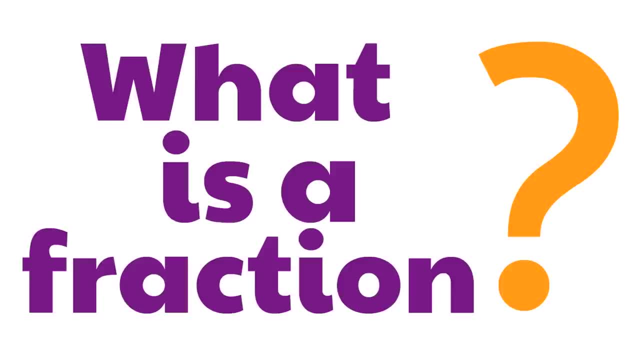 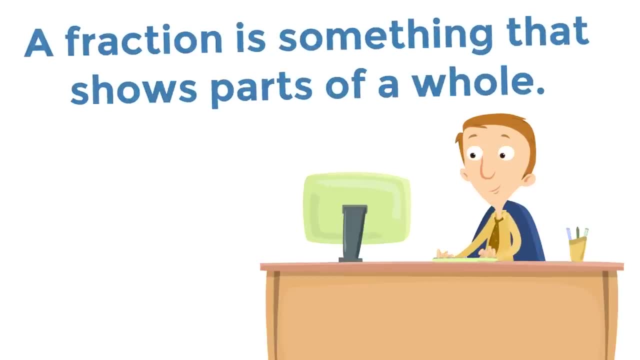 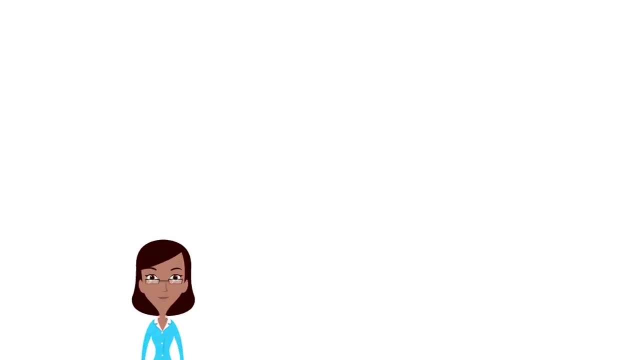 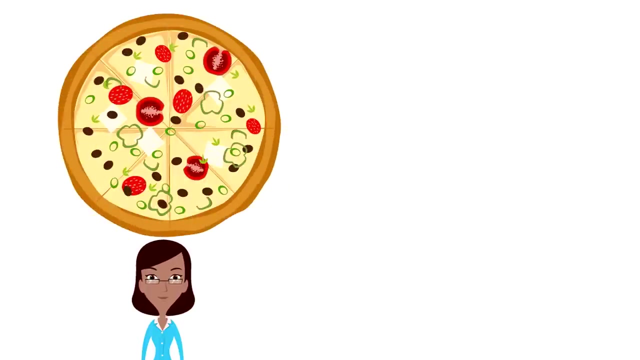 what do we mean? What is a fraction? Well, a fraction is something that shows parts of a whole. Let's say, there's this lady named Cindy. Cindy has a pizza, which is great. She loves pizza, So yummy pizza. But then her friend Chomsky arrives. 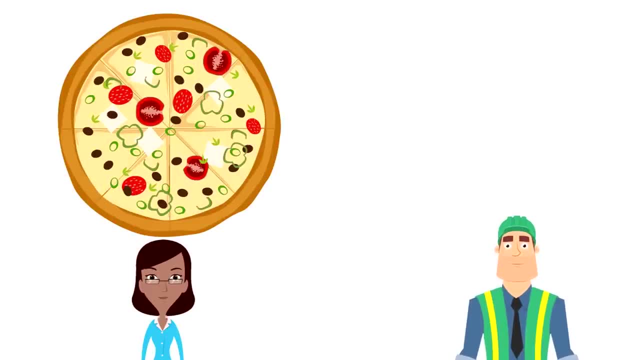 You remember Chomsky. Chomsky likes pizza too, and he's a little bit hungry. So maybe Cindy isn't going to eat the whole pizza now. Maybe they're going to split it, What do you think? So they split the pizza in half. 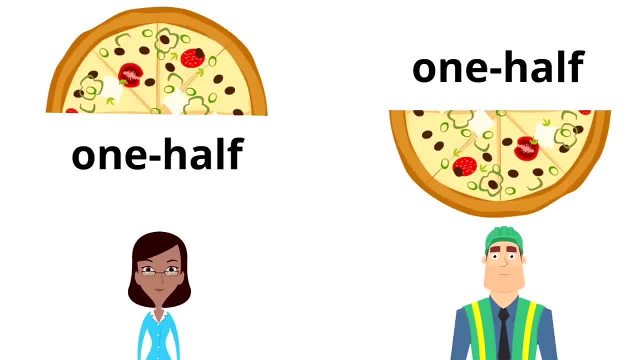 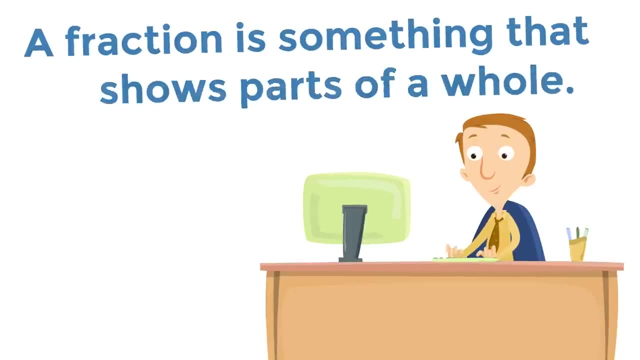 Each of them get one half of the pizza. Isn't that neat. Then everyone has pizza. Each of them have one half of the pizza. They split it right down the middle. Now remember, a fraction is something that shows parts of a whole. 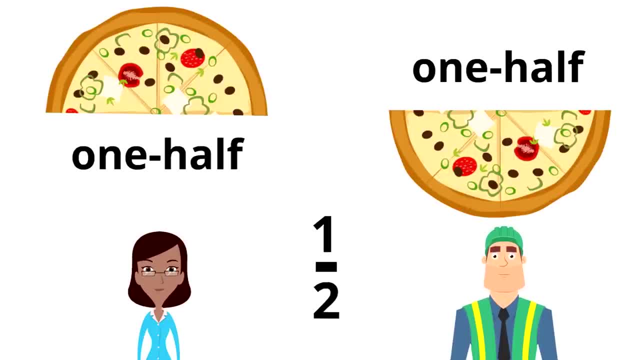 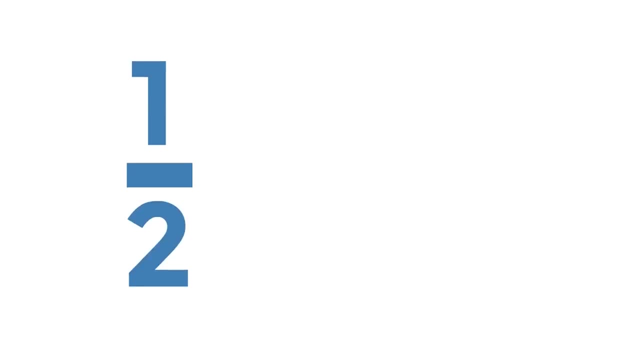 So here is what the fraction looks like: A one, a line and a two. That is the fraction, one half. Each of them- Cindy and Chomsky- get one half of the pizza, So this is one half. It's a very important fraction. 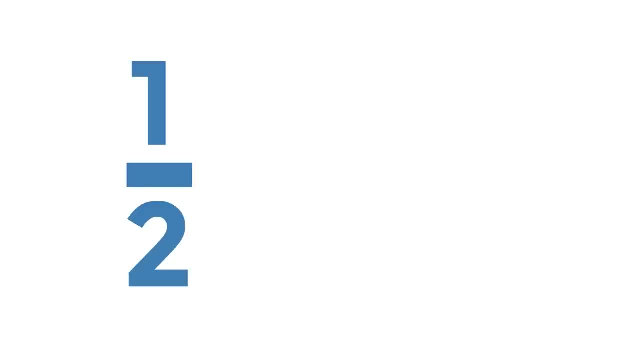 because we use it all the time. Now you might be wondering what do the numbers mean and how does it show one half? Well, the bottom number shows the total number of parts. The top number shows how many parts we are talking about. 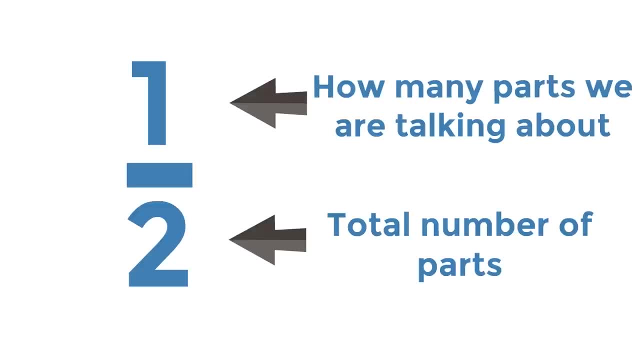 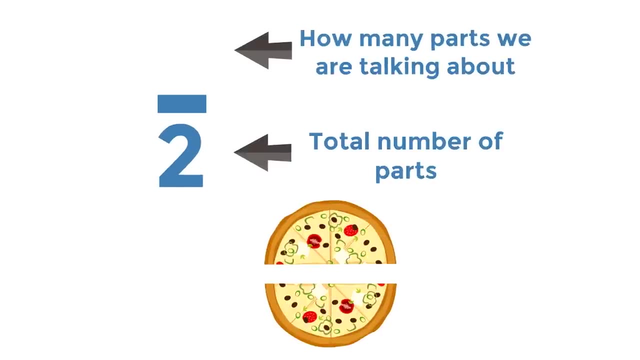 Pretty simple. Let's go back to our example. There are a total of two parts to the pizza. So there's a two on the bottom and Cindy just gets one part. That's the part we're talking about. So Cindy gets just one half of the pizza. 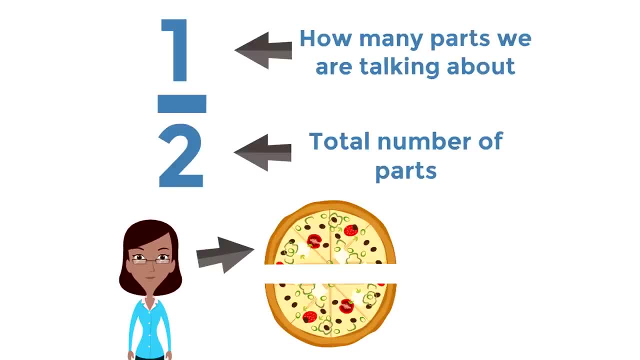 She doesn't get the whole thing, She gets just one part. She gets one half. The bottom number of a fraction is called the denominator. The denominator is the total number of parts. The top number is called the numerator. The numerator tells us how many parts we are talking about. 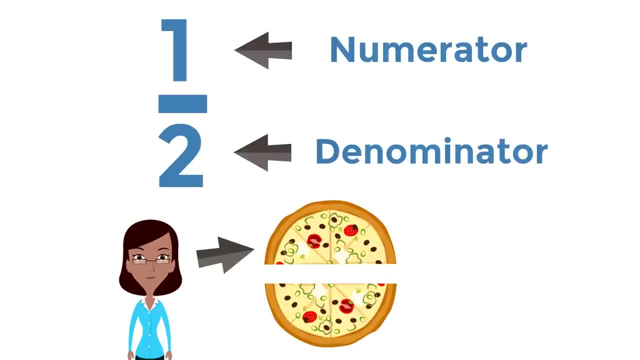 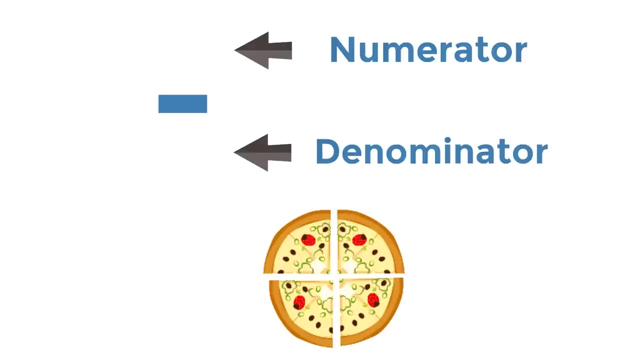 In this case Cindy is having one part of the pizza. The other part, of course, is going to Chomsky. Let's try this. Let's say there's another pizza and this pizza has four parts. The number four is the denominator. 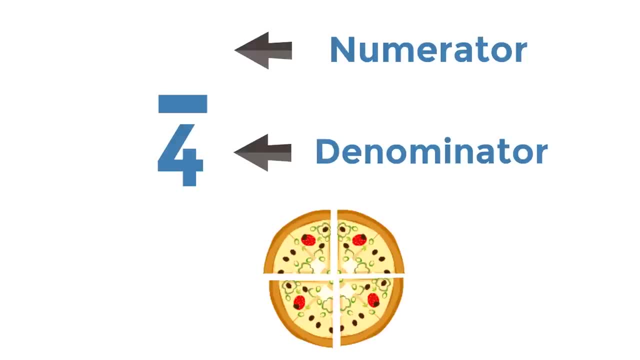 because there are four pieces of pizza, Four parts. Let's say Kelly shows up and wants to have one part of the pizza, one piece of the pizza, The numerator or the top number of the fraction is the number one, because Kelly is having one part or one piece of the pizza. 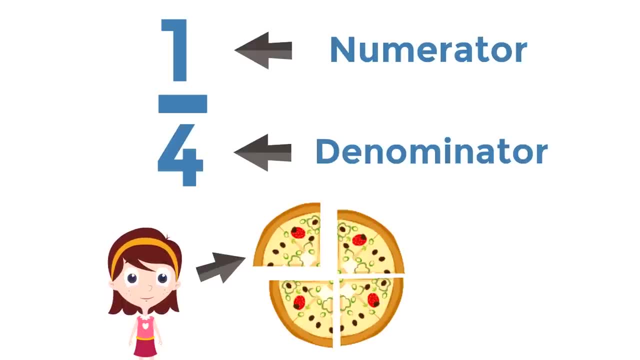 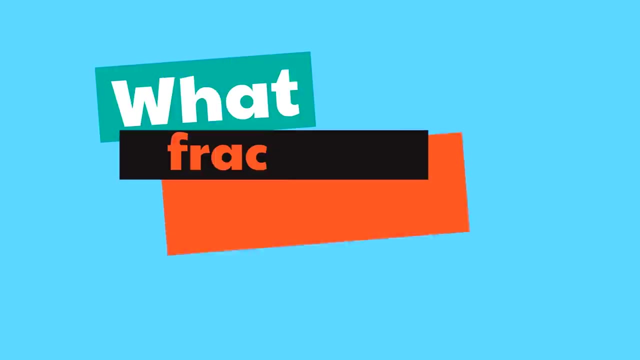 Kelly is having one fourth of the pizza. Pretty simple, Pretty fun. Fractions are awesome. Now we're going to need your help. Help us figure out what fraction is it. Huh, What fraction is it? Well, we're going to have a great time. 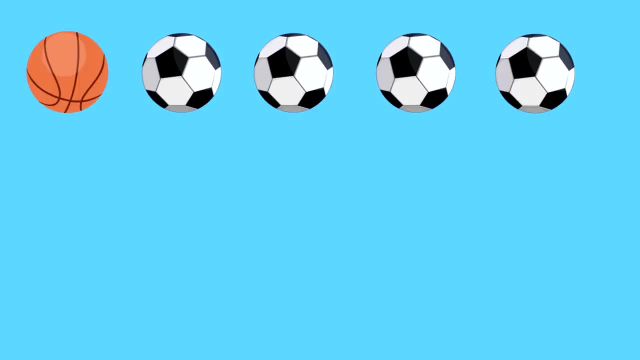 Let's say we have a group of five sports balls. One is a basketball, The other four are soccer balls. Let's figure out what fraction of the balls are basketballs, What fraction of the balls are basketballs. So we know a fraction has a line in the middle. 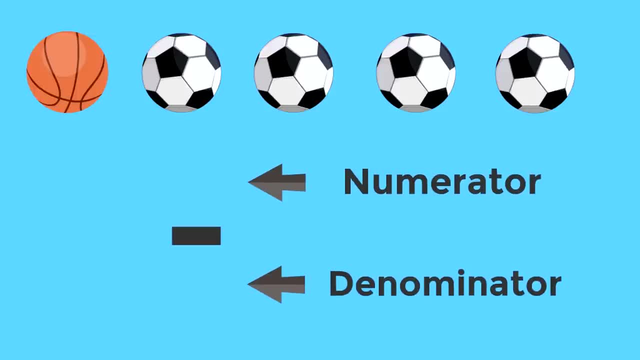 and the top number is the numerator and the bottom number is the denominator. The denominator shows us the total number of parts or units. How many sports balls are there? Yeah, Five, Five is the denominator. Good job, Now remember, we're asking for the fraction of sports balls. 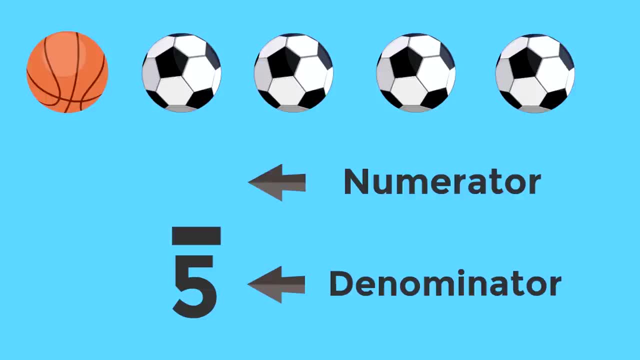 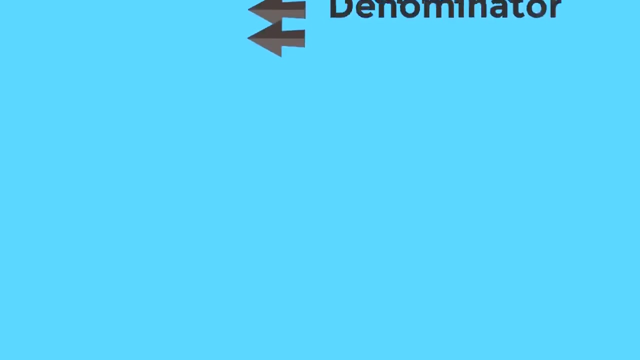 that are basketballs. So how many basketballs are there? Yeah, Just one. The number one is the numerator. So one fifth of the sports balls are basketballs. One fifth, Great job. Let's try this final example. Let's say there are five pets. 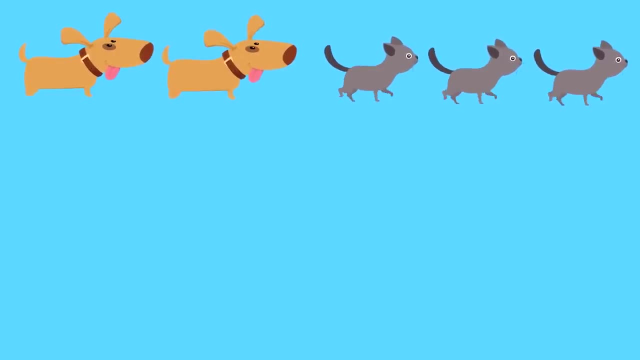 Five pets. Two of them are dogs and three of them are cats. What fraction of the pets are cats? Huh, That's a good question. What fraction of the pets are cats? Remember, here's what a fraction looks like. It's got a line in the middle. 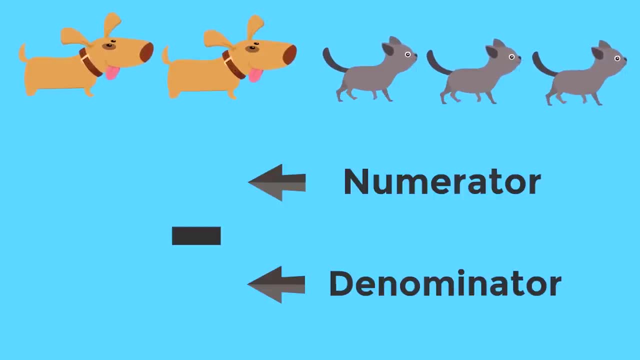 with the top number being the numerator and the bottom number is the denominator. So the total number of pets is five. What number is the denominator? What number goes on the bottom? Yeah, Five, Five is the denominator. It tells us the total number of pets. 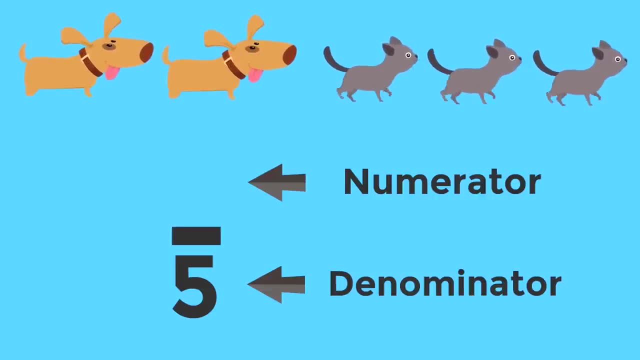 Remember, we're asking for the fraction of the pets that are cats. How many cats are there? Yeah, Three. So what's the numerator? Yeah, Three, Three is the numerator. Three fifths of the pets are cats. Wow. 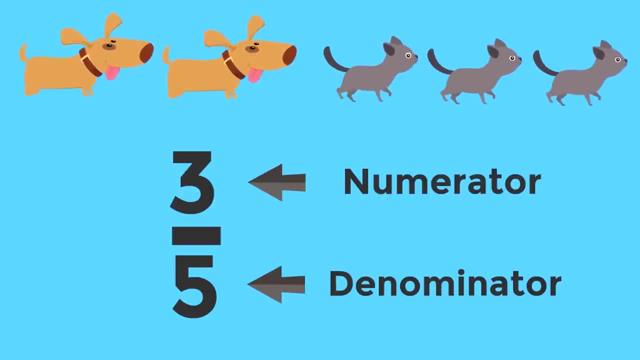 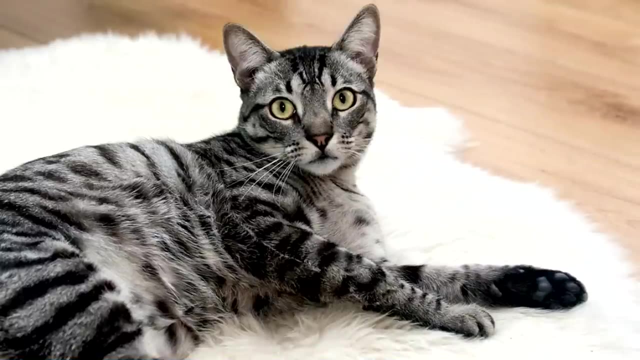 That was so cool, But none of those cats are as special to me as you, Mr Whiskers. Not even a fraction of my heart belongs to you, My whole heart. I love you, Mr Whiskers, I do. 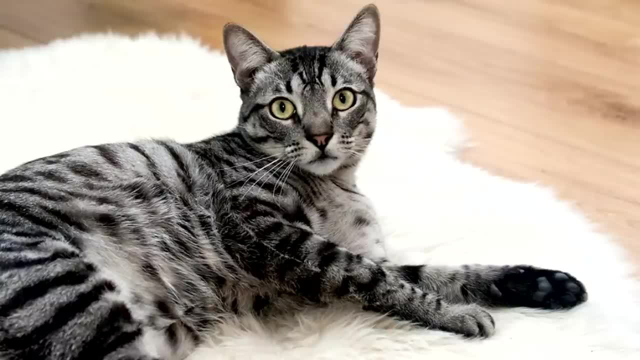 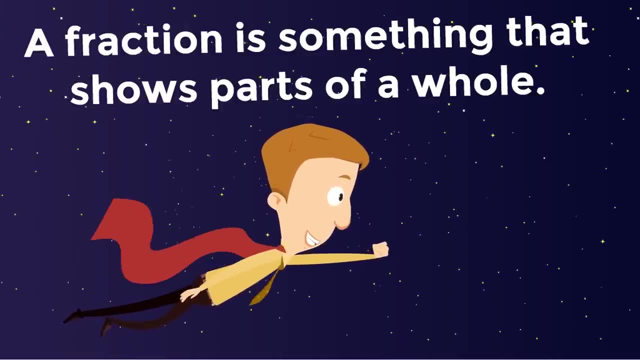 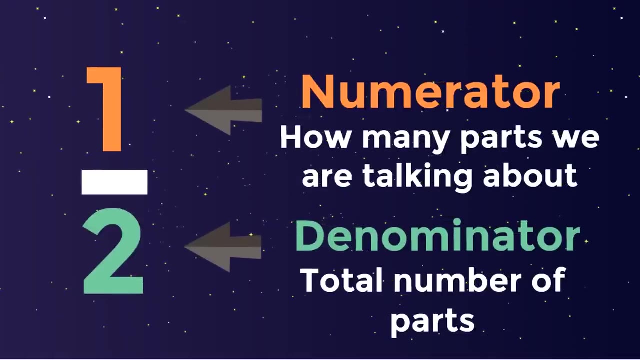 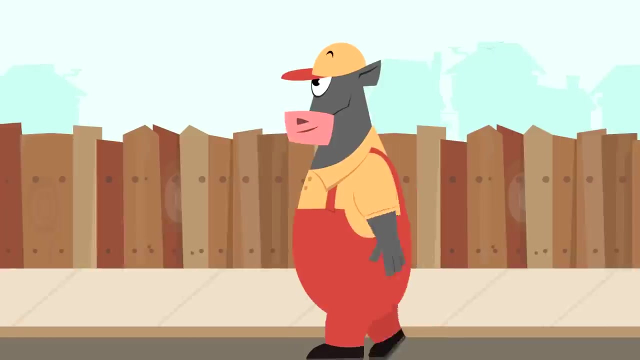 I do. A fraction is something that shows parts of a whole. The top number of a fraction is the numerator- how many parts we are talking about. And the bottom number of a fraction is the denominator- the total number of parts. Oh wow. 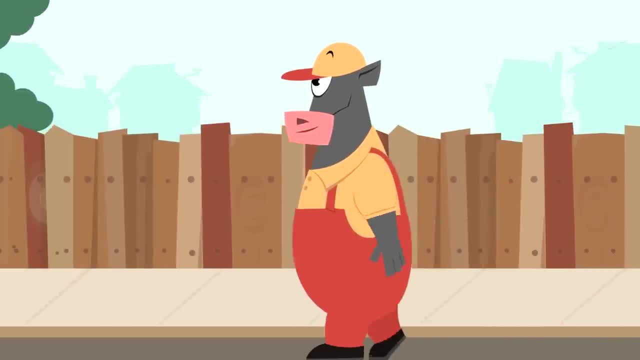 Look, It's the Homophone Cow. Homophone Cow, Homophone Cow. You're just walking, You're just going to ignore me. Well, I see how. it is Okay, so you're upset that we haven't included you in other videos. 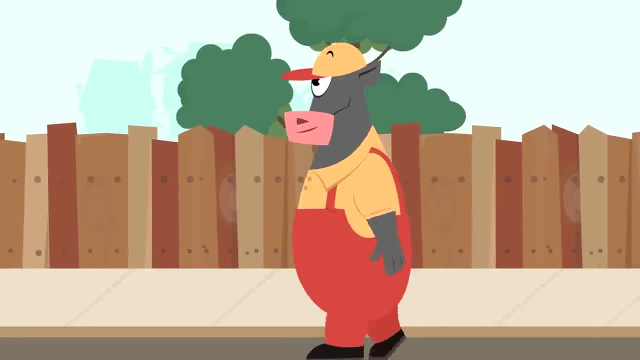 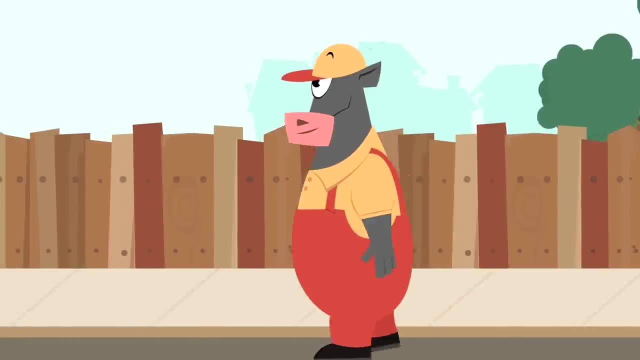 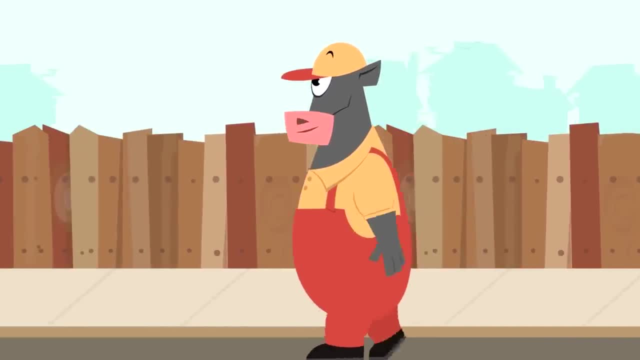 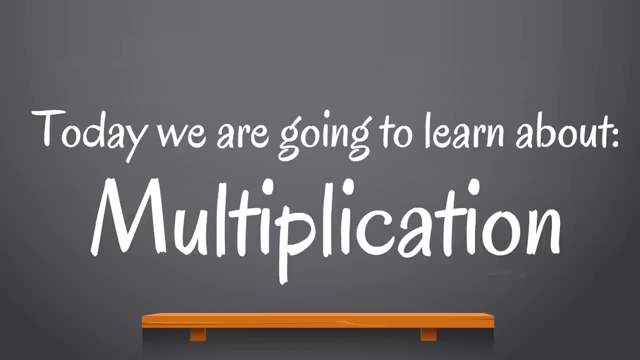 So, alright, I need to talk to the homophone cow, But in the meantime, let's learn about multiplication. You're going to learn how to multiply, And if that sounds really scary or if that sounds like a difficult thing, it's just because you don't know how to do it yet. 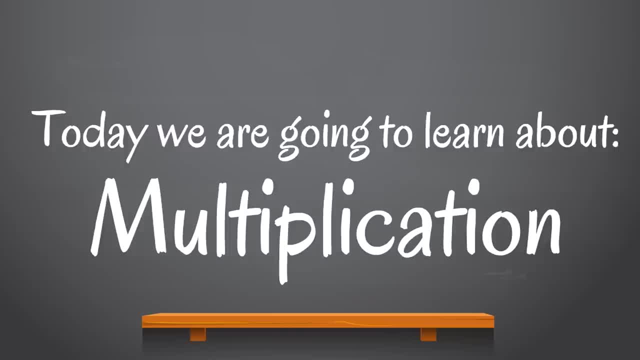 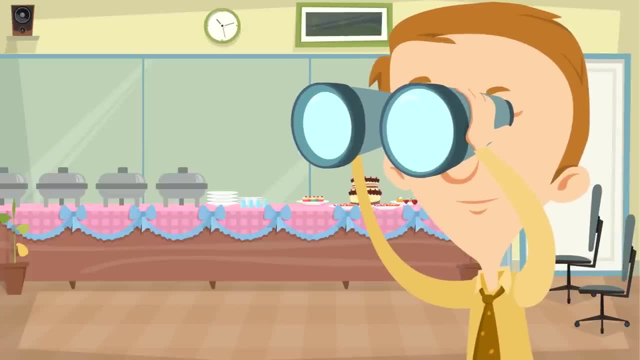 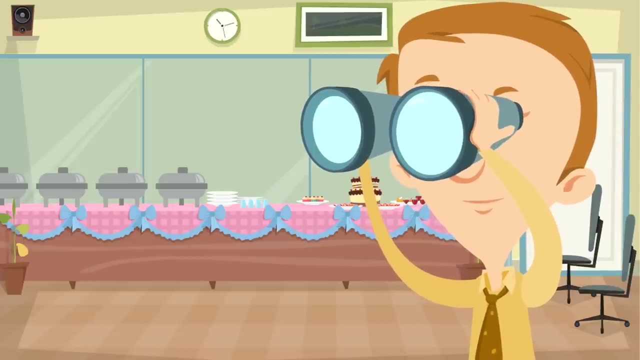 Once you learn the game, once you learn the process, it's fun, it's awesome. You see, multiplying is like being a detective: You're cracking a code, which is so cool. You're solving mysteries- like legit mysteries, Like I'm in an office building right now. 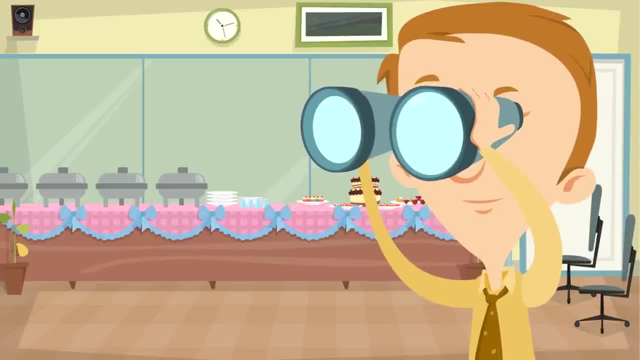 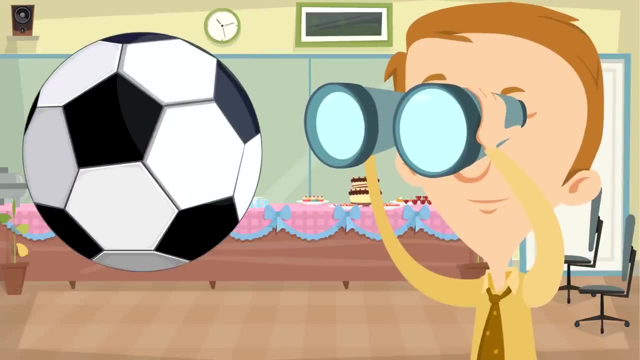 There's a cake behind me, For some reason. I'm looking out right now at you guys and I see that you're like whoa. we're going to multiply And once you learn it, it's just a game. So buckle in for the fun and the learning. 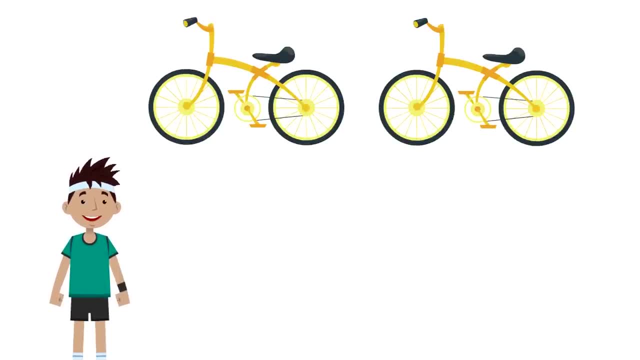 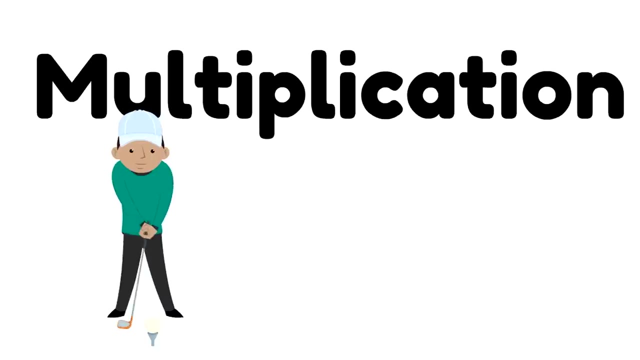 Let's say you have two bikes and for some reason they look the exact same, And somebody wants to give you an air pump. They ask a simple question: How many tires do you have to take care of? To figure that out, we're going to use multiplication. 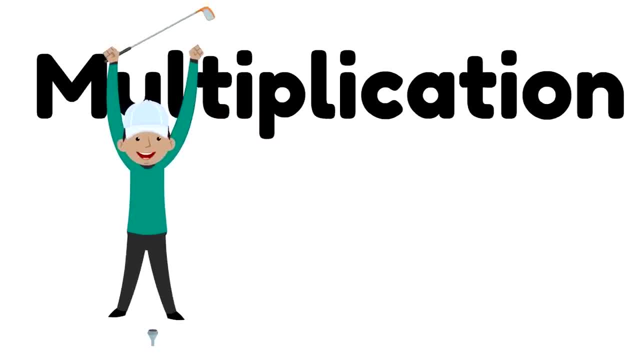 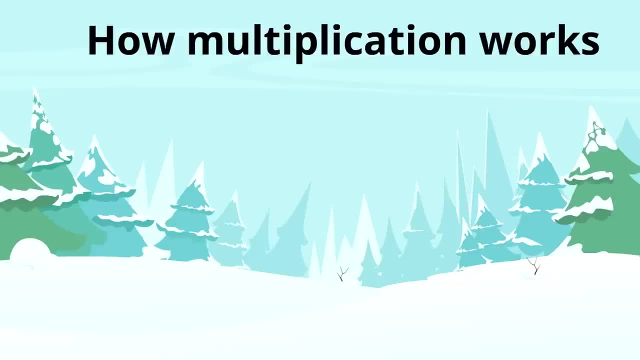 We're going to play the game. It's going to be awesome. Okay, so here is how multiplication works. So we put the number that's in each group, and then we put this X, which means times, and then the number of groups. 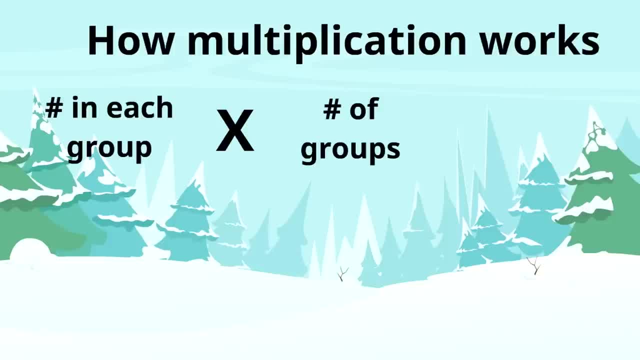 So that tells us how many times that number is going to show up, and then we add them all together and you've got your answer. Isn't that cool? And just a side note: to work there has to be the same number in each group. 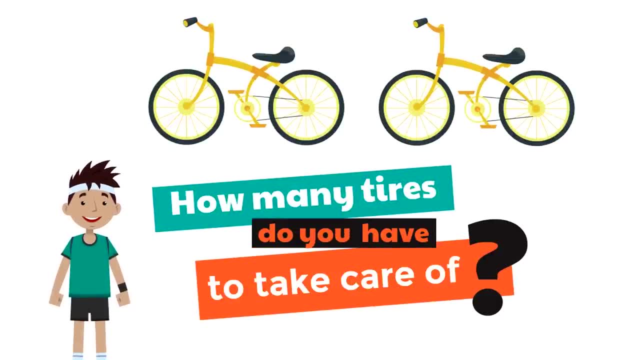 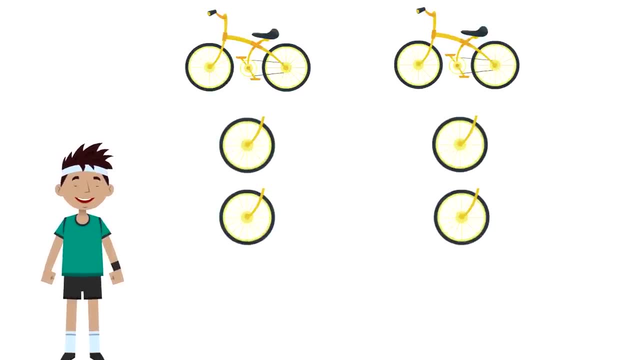 Now remember, we're trying to figure out how many tires you have to take care of if you have two bicycles. All right, now we have the wheels under each bike. Each bike has two wheels, One, two, So we write down a two. 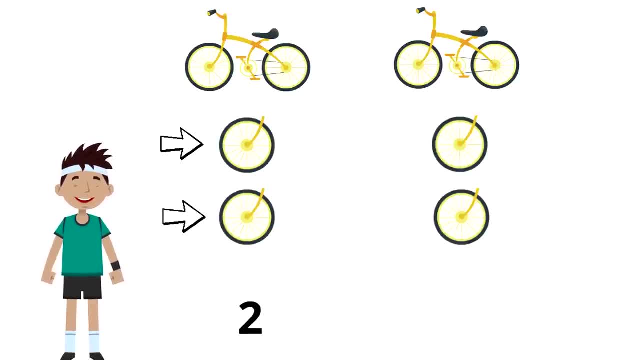 Each bike has two wheels. Remember, the first number we write down with multiplication is the number in each group. Then we write an X. This X means times Two times. It's the symbol of multiplication. All right, the second number we write are the number of groups. 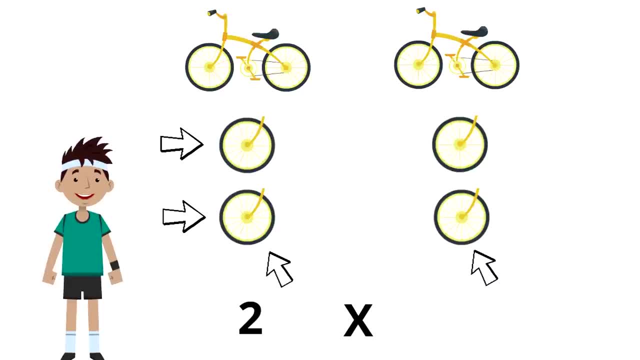 You can see them here. How many groups do we have of two? How many, Yeah, two. So it reads: two times two. To figure this out, we are going to skip count by two. Two, four. That means two times two equals four. 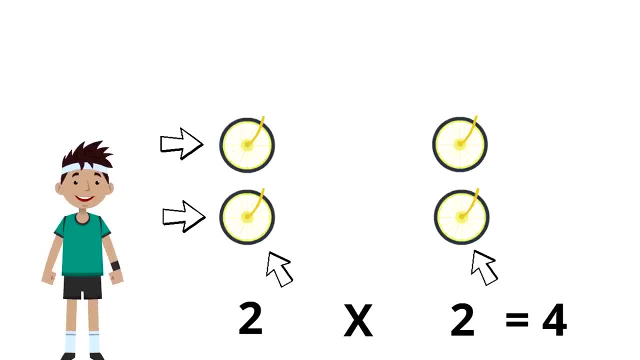 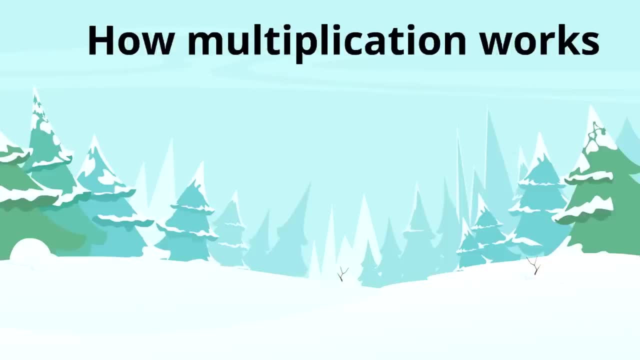 If you have two bikes, that means you have four wheels. Two two times is four. Remember this is how multiplication works: The number in each group times the number in each group. The number in each group times the number in each group. 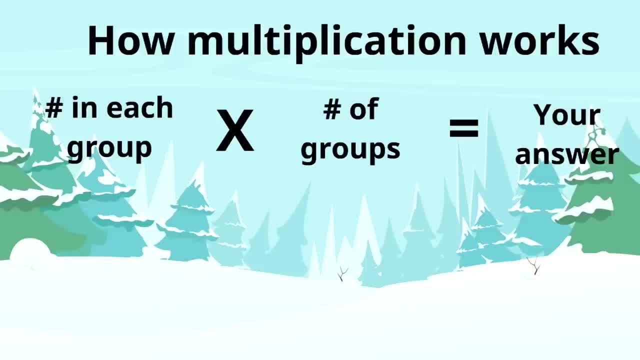 The number in each group times the number in each group. I'm going to put together two things. Number in each group is the number of groups. The number of groups equals the answer. To learn byaya, you have to student how you File. 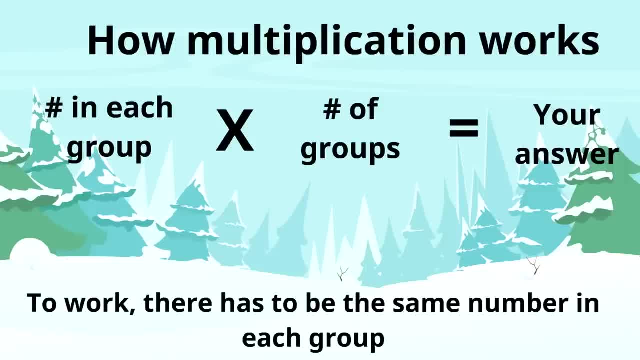 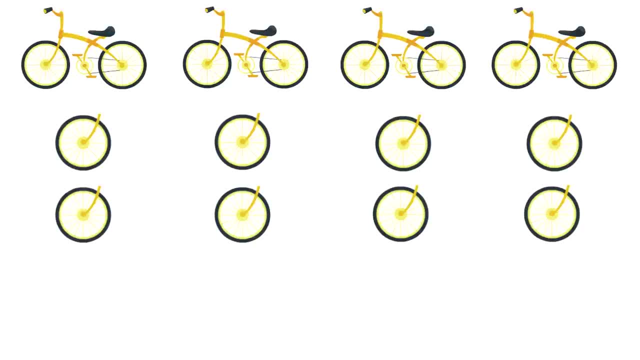 Alright, let's take this to the next level. Let's say somebody has four bikes. Here are their wheels. Whoo hoo, yeahhhh, You know how to do this. Each bike has two wheels, So the first number we write down is 4叫 4.. 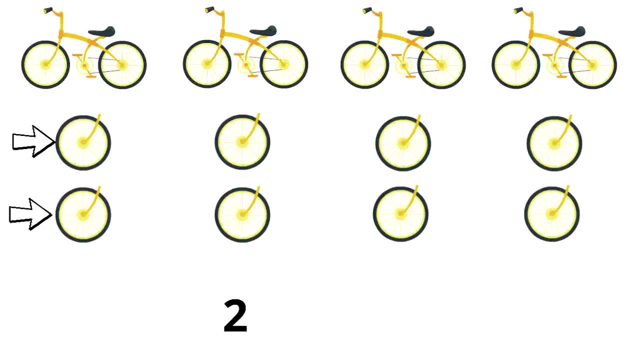 So now we have four is the number two. That's the number in each group. We're going to put the time symbol there and count the number of groups: One, two, three, four. So it's two times four. This is so much fun. This is multiplication. Now let's skip count to get the answer Two. 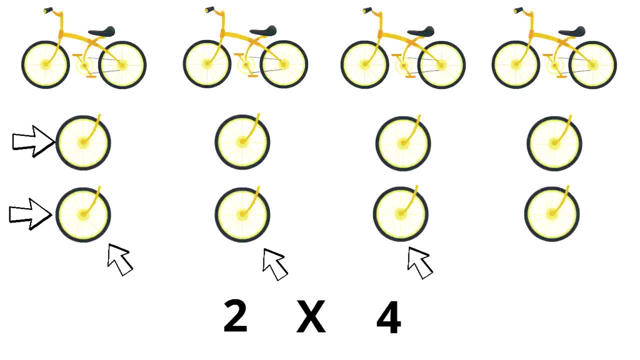 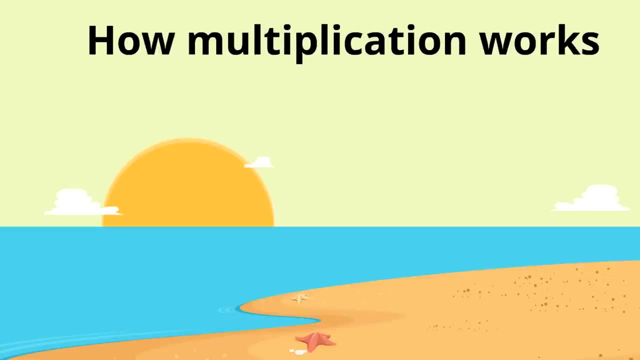 four, six, eight, Eight is our answer. There are eight wheels. Two times four equals eight. This is how multiplication works. We put the number in each group times the number of groups and we get our answer. You're getting the hang of it? Alright, let's try this one. 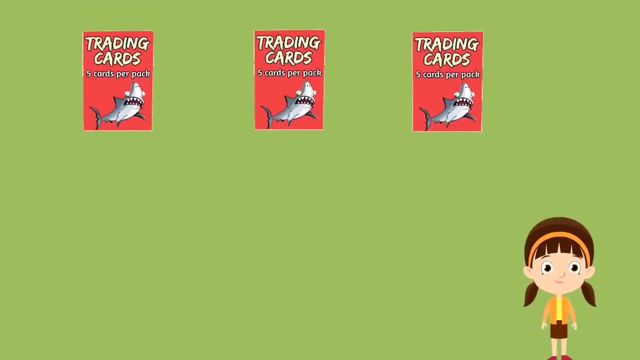 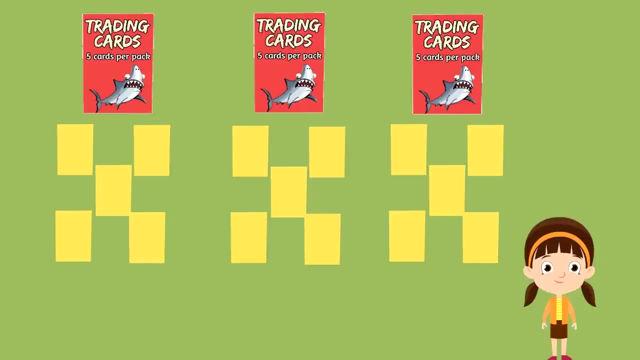 Okay, Let's say you buy three packs of trading cards. Let's say each pack had five cards in it. Huh, that's a pretty good amount. So three packs of five cards, How many cards did you get in total? That's a really great question. Sounds like we're going to need. 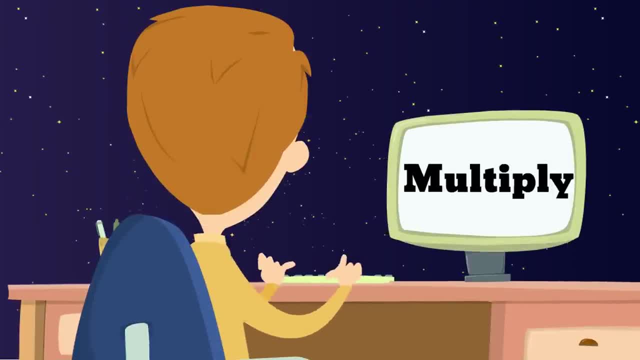 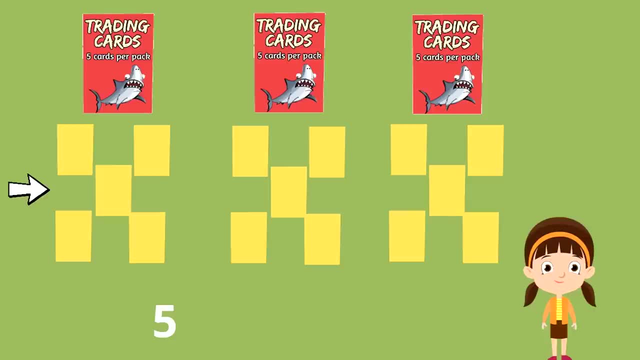 to multiply. So each group has five. So that's the first thing we write down: The number in each group, That's five. Put the multiplication sign, which is the x, which means times Five times How many groups are there? One, two, three. So the second number is three Five times. 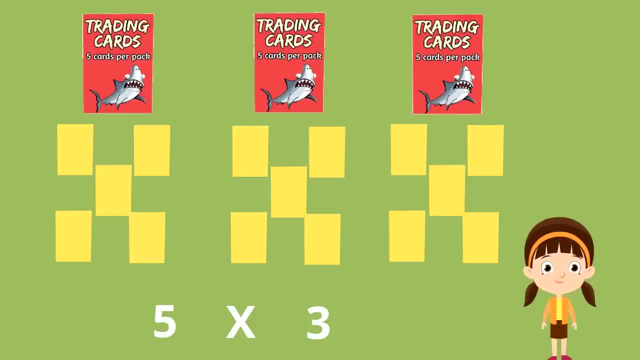 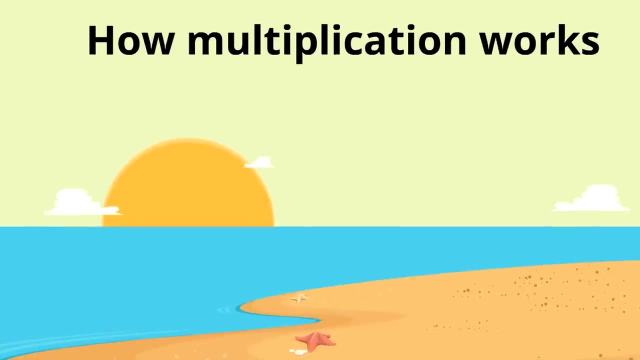 three. What's five times three? Six IS FIVE. find out: 5, 10, 15. 5 times 3 equals 15. you have 15 trading cards. all right, this is how it works. you take the number in each group, times the number of groups and you. 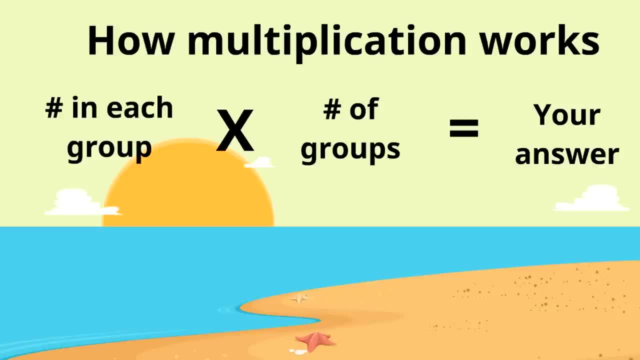 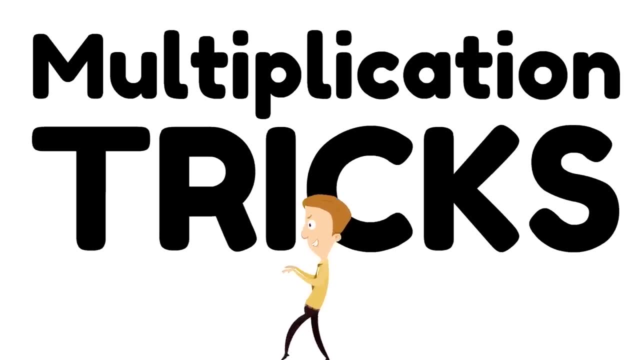 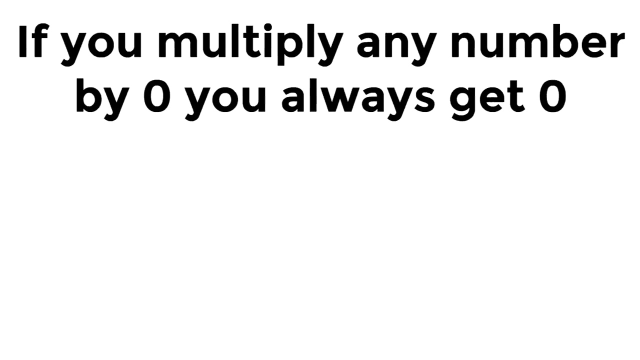 get your answer now. here are some multiplication tricks that are going to be really sneaky ways that you can figure out multiplication problems really, really quickly. here's the trick: if you multiply any number by 0, you always get 0. always, you always get 0. here's an example: 5 times 0. 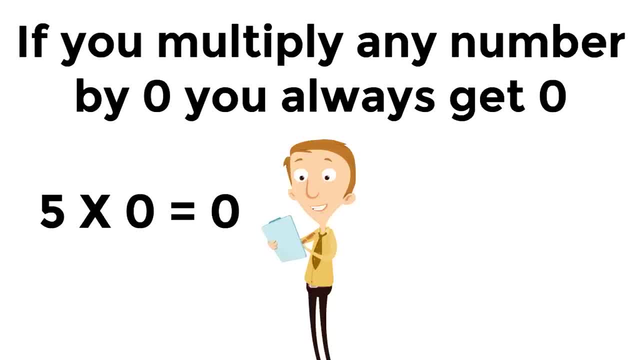 you always get 0. here's an example. 5 times 0, you always get 0. here's an example: 5 times 0 equals zero. when you have zero groups of five, that means you have zero. there are none. whenever you multiply any number by zero, you always get zero 100 times 0. 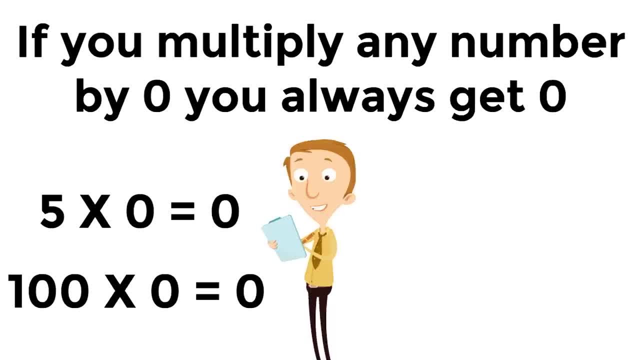 equals 0. even if 0 is the first number in the equation, you still always get 0. when you multiply by any number- for example, 0 times 11 equals 0 and 0 times 1000 equals 0- but if you multiply any number by 0, you always get 0. all this: 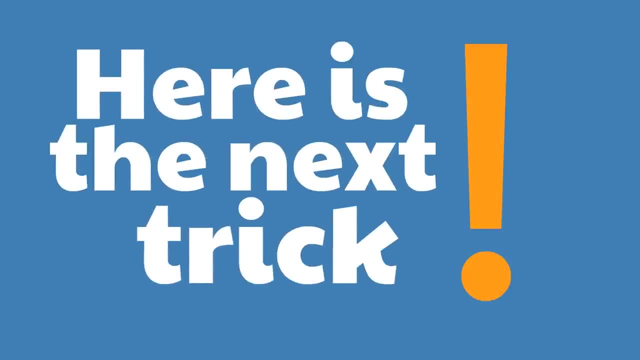 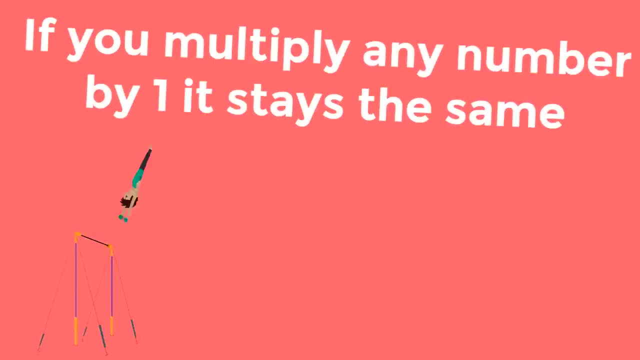 has been so much fun. here is the next trick. if you multiply any number by 0, you're gonna 0 equals 0. im just kidding. by 1 it stays the same. Look at these: 7 times 1 equals 7, 100 times 1 equals 100, 33 times. 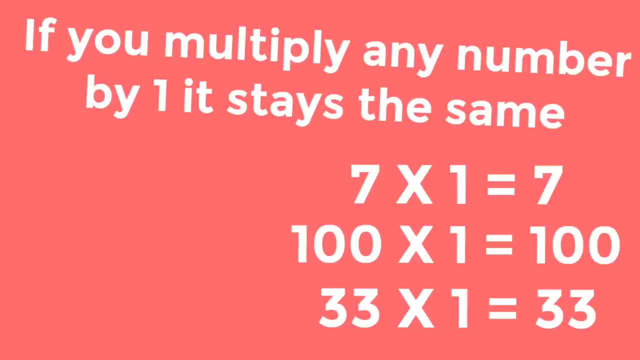 1 equals 33.. If you flip them, the answer stays the same: 1 times 7 equals 7, 1 times 100 equals 100, 1 times 33 equals 33.. Honestly, the order of the multiplied numbers does not. 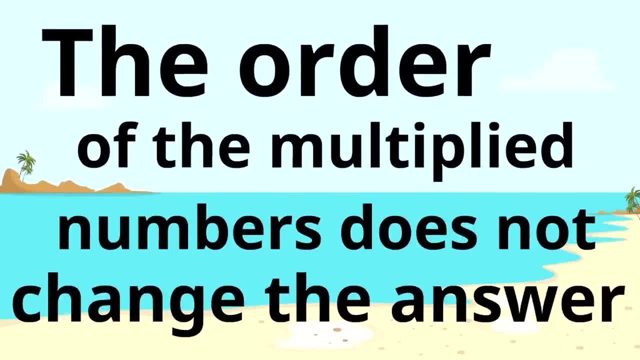 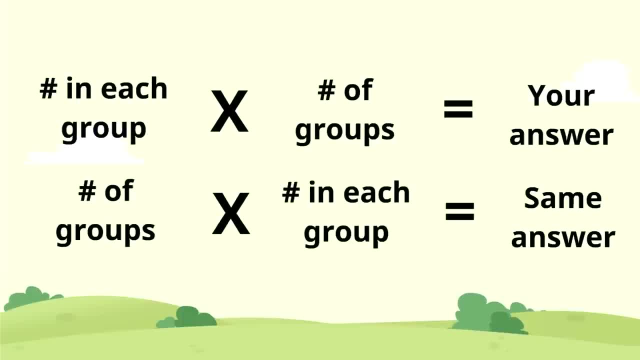 change the answer. If you were to flip the number of groups and the number in each group, you would still get the same answer, Though we still recommend this way. so simple: the number in each group times the number of groups to get your answer. So the two tricks have. 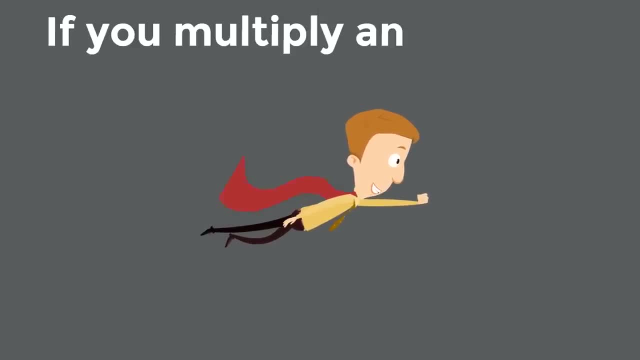 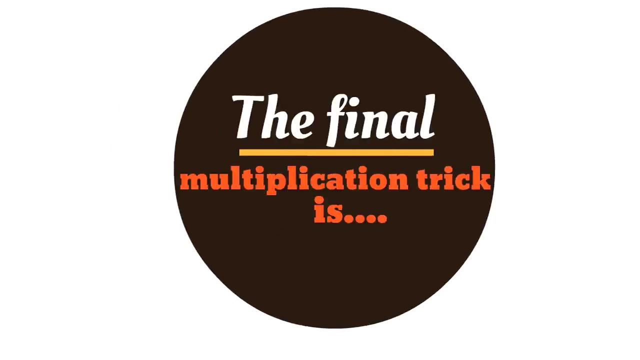 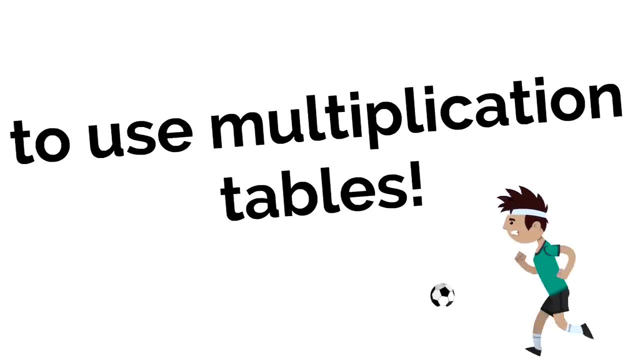 been. If you multiply any number by 0, you always get zero, and if you multiply any number by one, it stays the same. the final multiplication trick is to use multiplication tables. they come in all shapes and sizes but they are all helpful, especially as you're first. 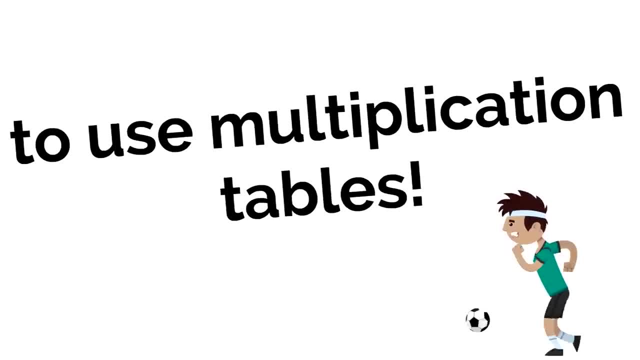 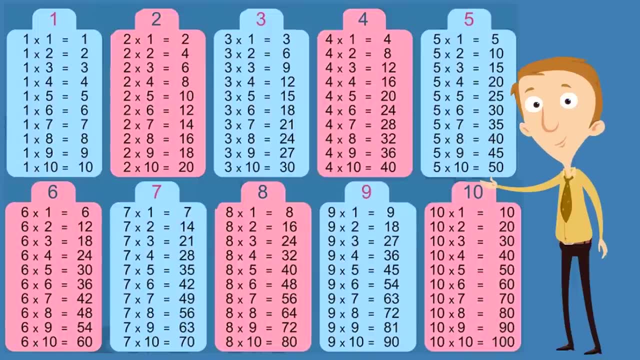 learning how to multiply. here are some examples of multiplication tables. there's a table for all of the numbers from 1 to 10. some kids memorize tables like these so that they'll know right off the bat in a moment what an answer could be for certain multiplication problems. this is how multiplication 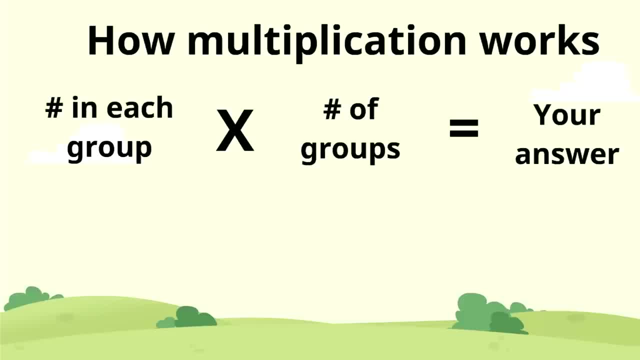 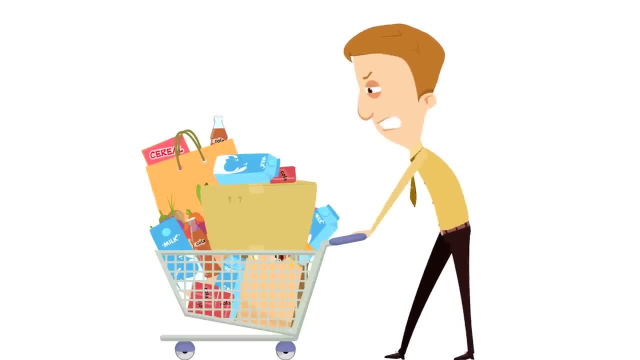 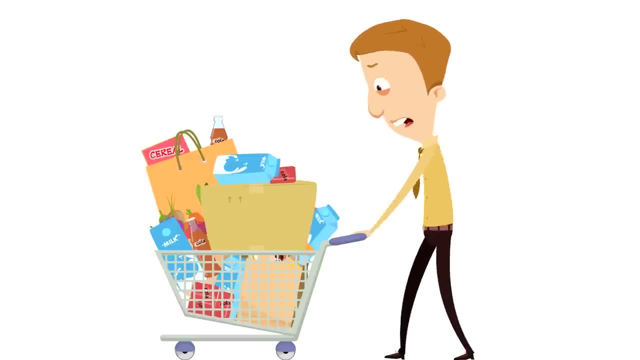 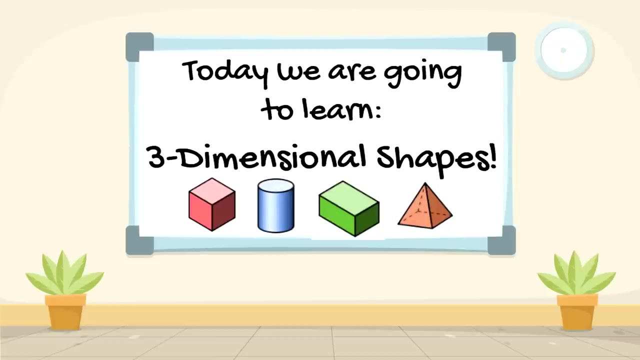 learning fun, so that learning isn't hard like pushing this cart. oh my goodness. all right, what's the next thing we should learn about? let's learn about three-dimensional shapes. this is going to be awesome. love the 3d shapes. a lot of people though the 2d shapes. you might not know the 3d shapes- you're in the. 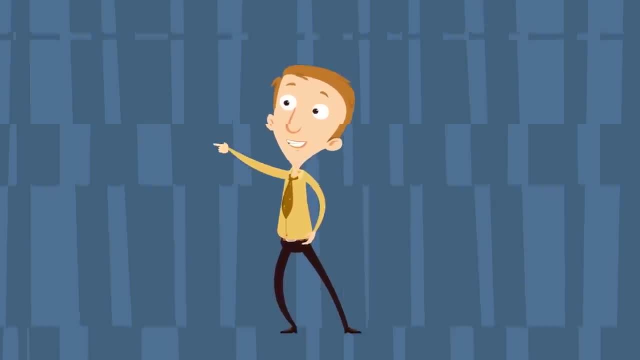 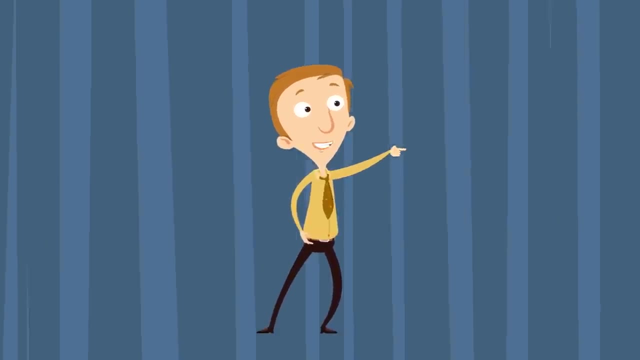 right place. before we get started, you just dance here real quick. this is really cool music. I really like this it's. you know some people. they're not dancers. I dance side dabble and dancing alright, alright. can somebody turn that music off from to? alright, that's enough. 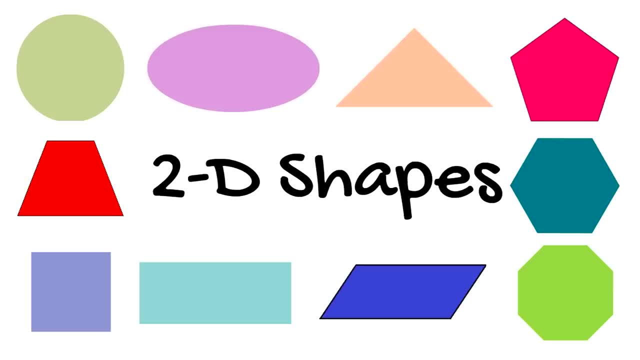 Can somebody turn that music off? I can't teach like this. I can't teach with this music going on. I feel like I'm in a candy shop. Let's just start the music off, please, Thanks. So here they are, our old friends, the 2D shapes. You're familiar with these, you know. 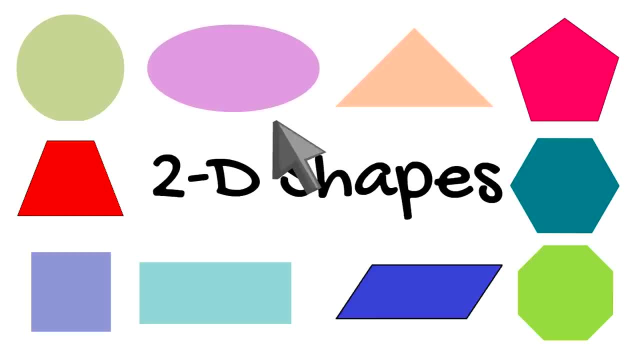 You're familiar with the circle, the oval, the triangle, the pentagon, the trapezoid, the hexagon, the square, the rectangle, the parallelogram and the octagon. These aren't all our shapes, our 2D shapes, you know. 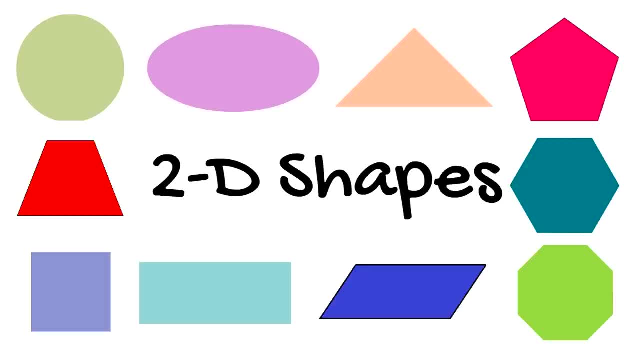 But these are old family friends of ours. We don't want to just forget about these, And before we look at 3D shapes, it's really important for us to look at these shapes again because these are old friends. So we're going to look at each one of these one by one. 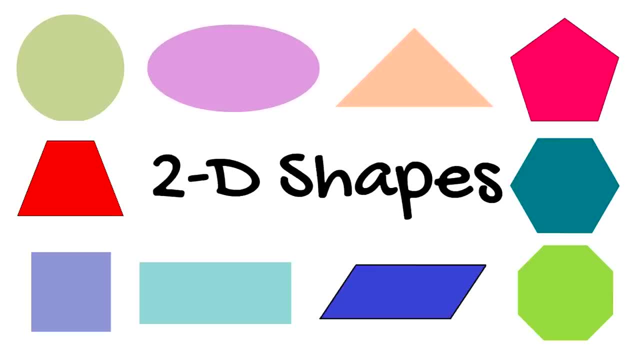 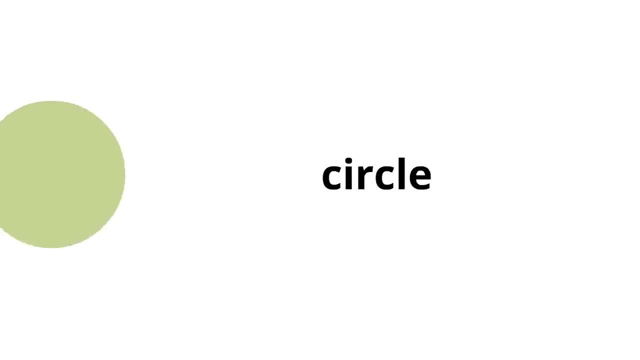 just to make sure you know who they are before we learn all these new shapes. This first shape doesn't even need an introduction. It's the circle. the circle, that round figure. It's awesome. We love this shape. It's one of the first ones we ever learn: the circle. 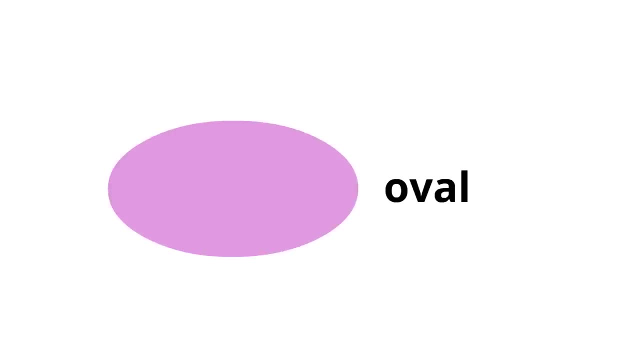 This next shape is one of the stretchy shapes: the oval. It's like a circle got stretched out, It's elongated. It's a tremendous shape, the oval. Here's another familiar shape: the triangle. three sides. We love the triangle. The triangle is great. The three-sided friend. three sides, a triangle. 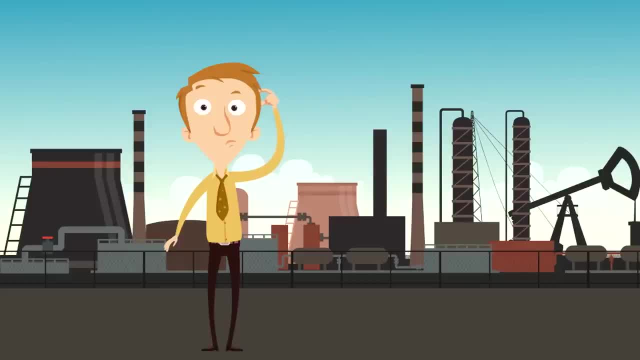 Wait, I keep saying we love the shapes. I mean we like the shapes, but do you love the shapes? Do I love the shapes? I mean, I don't know, Maybe I need to take it easy here. All right, let's keep going. 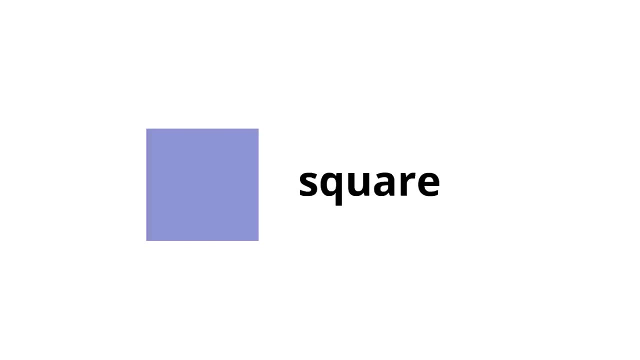 Ah, the square. four sides, all equal. You know, the square's good, The square's a good shape. you know, Sometimes you just need a square, Sometimes you just need a square. Here's the rectangle. The rectangle is longer than the square. 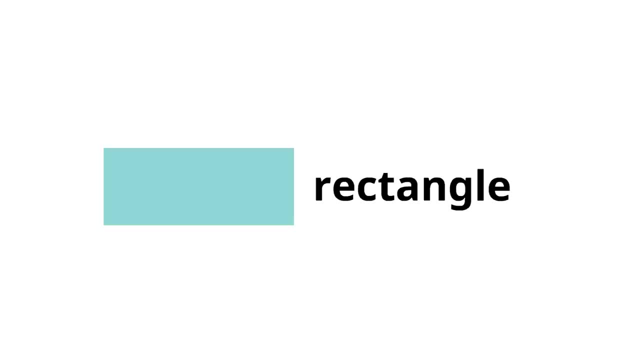 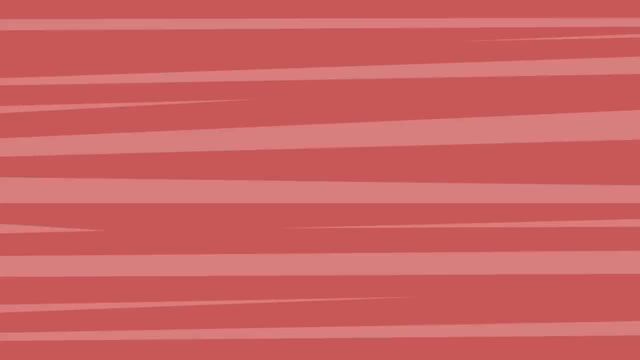 because not all four sides are equal: The rectangle. I know, I know, I know We're in the middle of something here, but I have to share this again. So what do you call a hamster with a top hat? 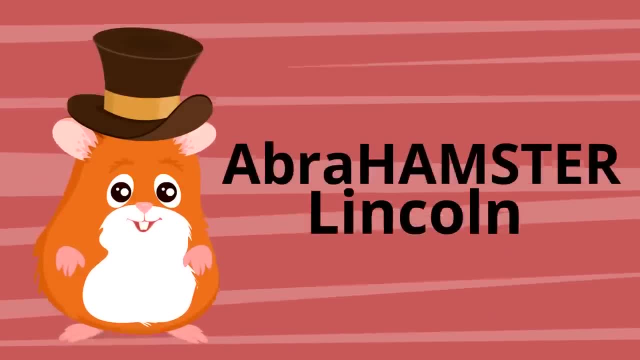 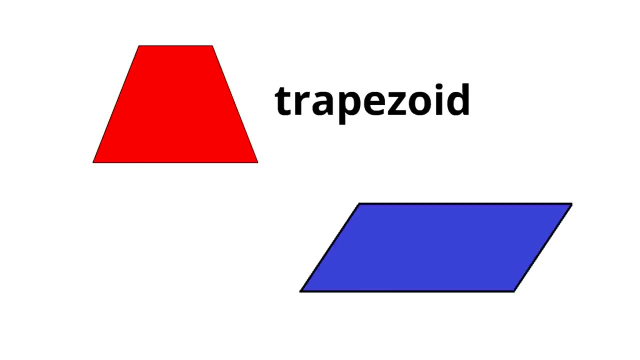 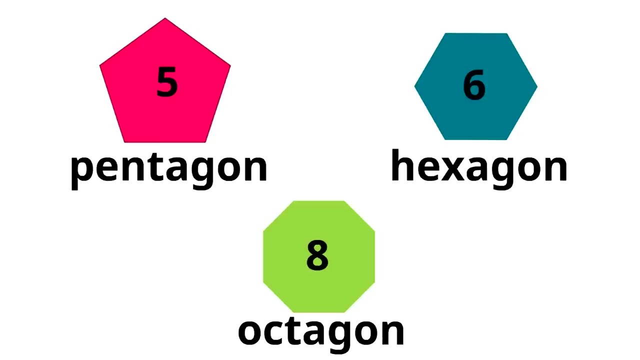 Abrahamster Lincoln. I digress. The trapezoid, a cool shape with two of the sides being parallel to each other, and the parallelogram, another four-sided shape. Both pairs of sides are parallel to each other. And finally, the pentagon with five sides, the hexagon with six sides. 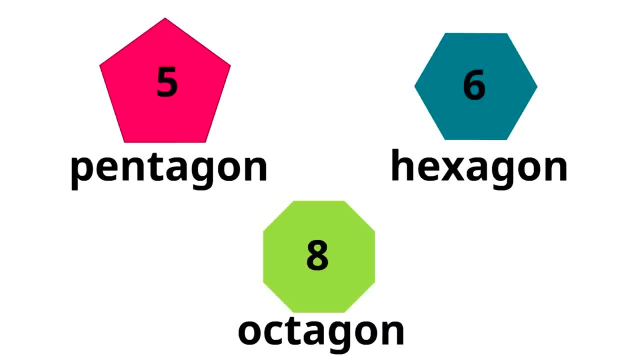 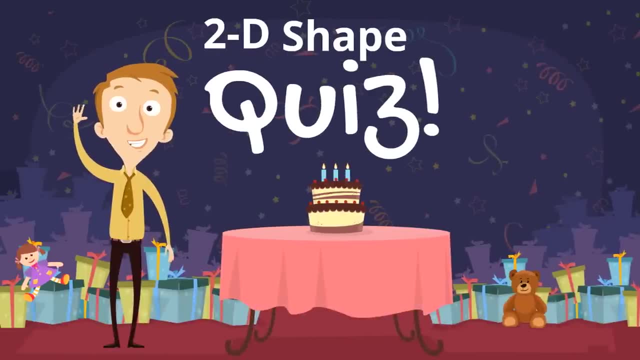 and the octagon with eight sides. What awesome shapes. So let's go ahead and do a quick 2D shape quiz. I need your help. I want to see if you really learned these, if you really know these, before we get into the 3D shapes. 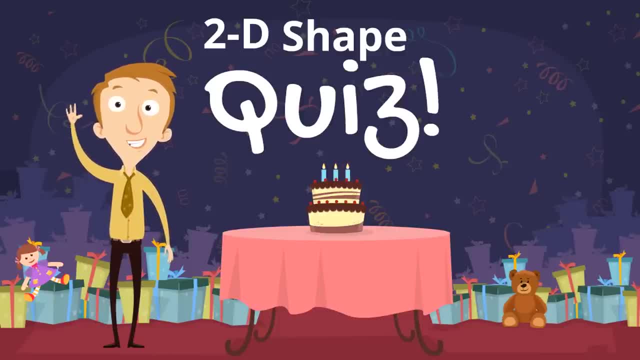 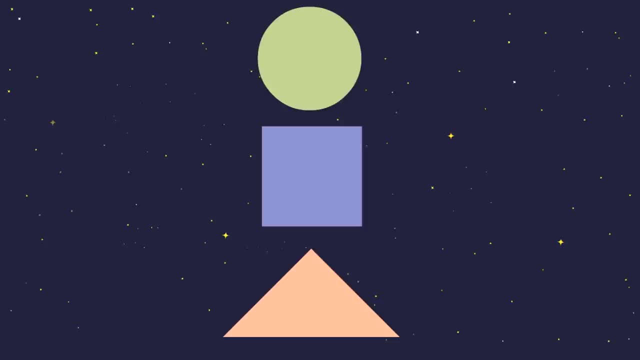 So help me out here. We're going to have an awesome time. Wait, what Is that? my birthday? Oh well, What type of shape is on the top? Yeah, a circle. What type of shape is in the middle? 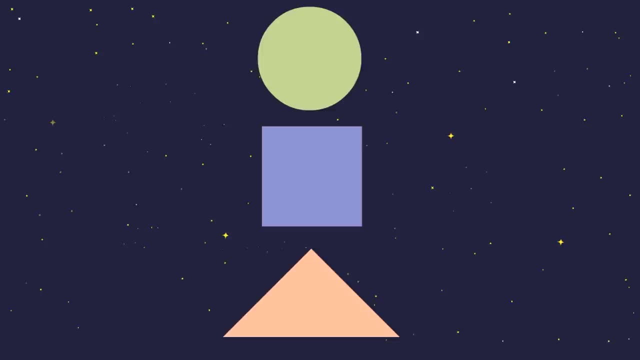 A square- Awesome, Okay. Now what shape is on the bottom? There's a square. What is the bottom? There's a square- Awesome, Okay. Now what shape is on the bottom? There's a square- Awesome, Okay. Now what shape is on the bottom? 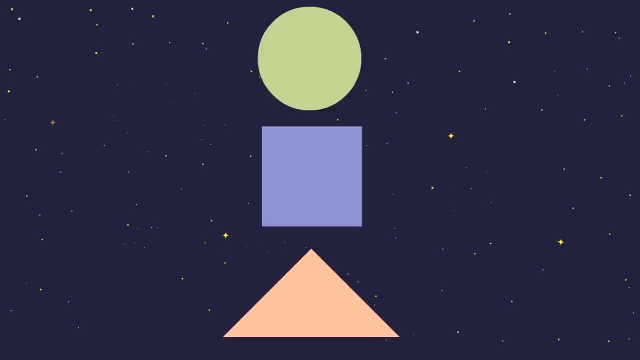 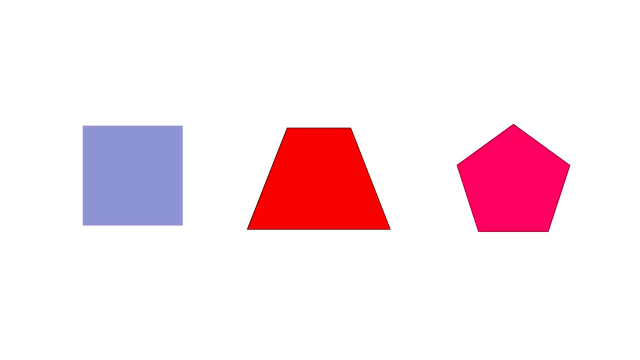 of course, a triangle. awesome job. now we've got more. this is a little trickier. which shape is in the middle? yeah, a trapezoid. which shape is on the right- the Pentagon- good job. and which shape is on the left? yeah, the square. now try. 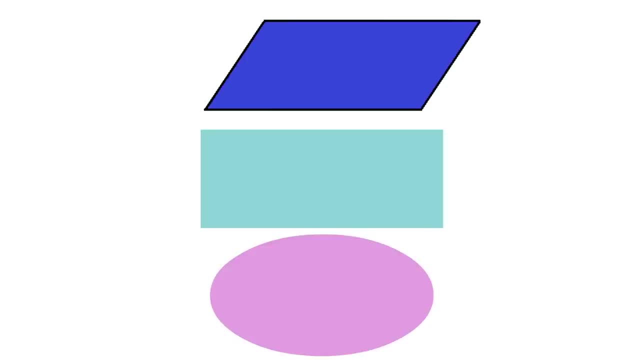 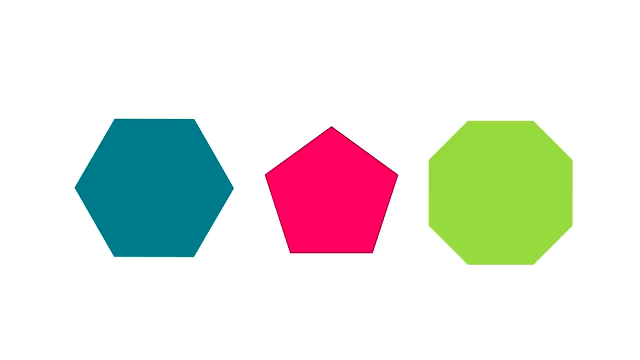 these? which shape is on the bottom? yeah, the oval. which shape is on the top? yeah, the parallelogram. which shape is in the middle? all right, the rectangle, great job. all right, the last one. which shape is on the left? yeah, the hexagon. which shape is on the right? 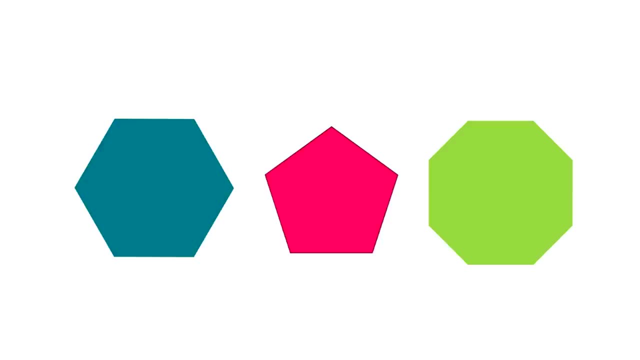 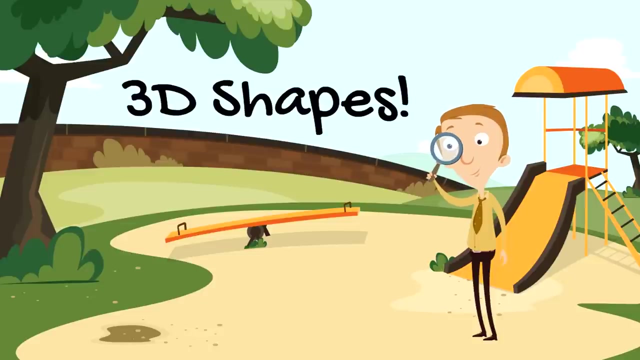 great, the octagon. and which shape is in the middle phenomenal- the Pentagon? all right, we're ready to learn the 3d shapes. we're gonna learn how to identify the three-dimensional shapes. if you struggle through the quiz, you might want to watch the first part of the video. 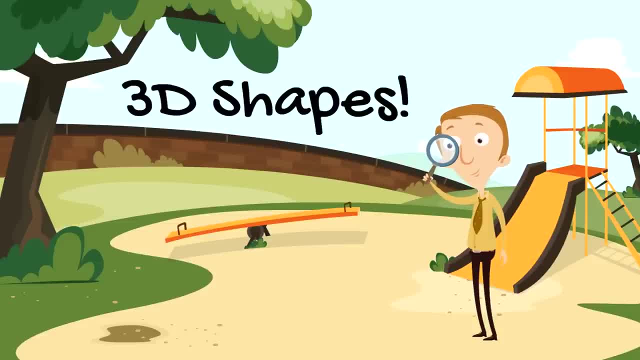 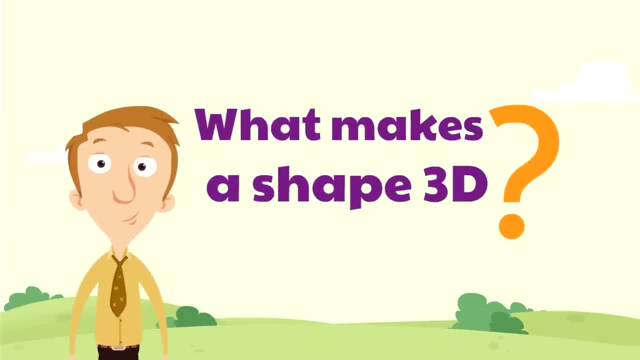 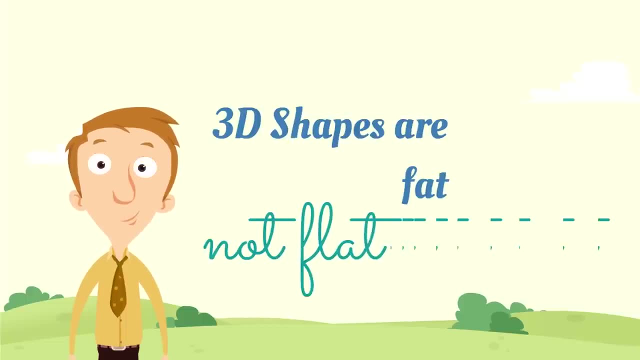 again, otherwise let's get started, get started. so, as we're starting out, it's important to remember what makes a 3d shape of 3d shape. there's an old rhyme that says 3d shapes are fat, not flat, and you can see that with the sphere, which is a 3d shape, we're about. 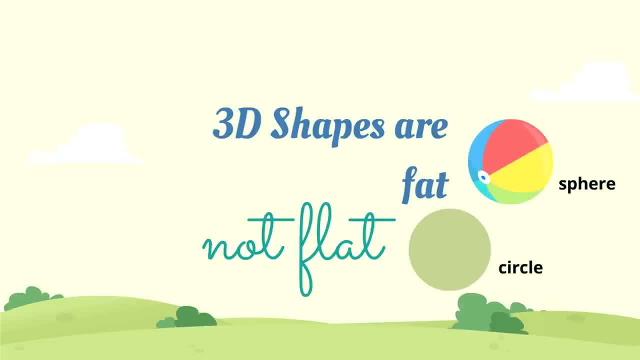 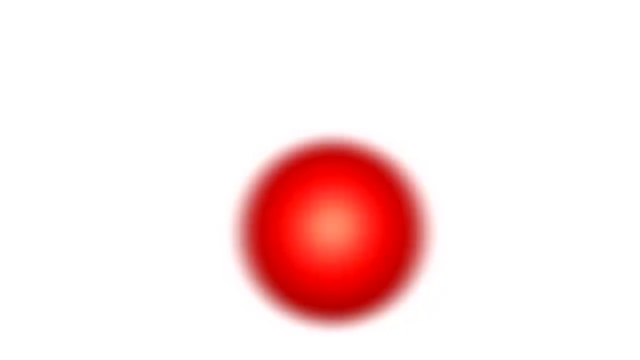 to learn and the circle. the circle is flat, but the sphere is 3d, it's three-dimensional. all the shapes are like that, so let's learn all these 3D shapes. So the first 3D shape we're going to learn is the sphere, The one that 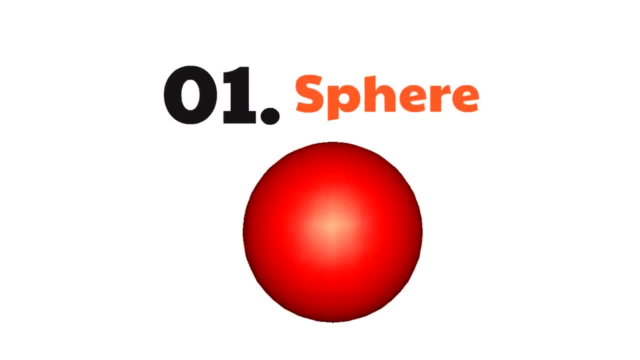 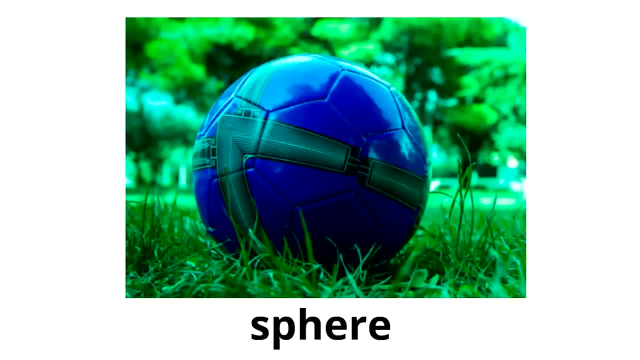 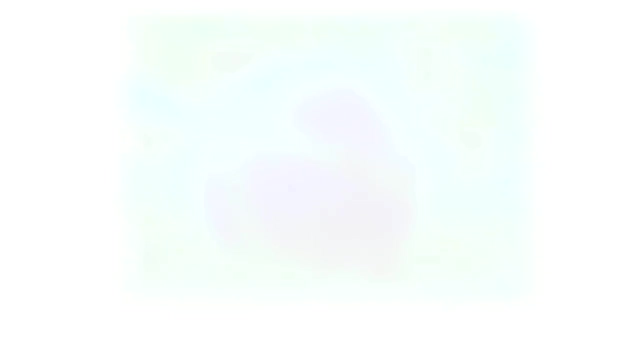 we just mentioned. the sphere is the 3D version of the circle. It's perfectly round. There are spheres all around us. One of the spheres we see all the time are balls like this soccer ball. A soccer ball is a sphere, It's perfectly round. It's a 3D circle. It's a sphere. You know this. 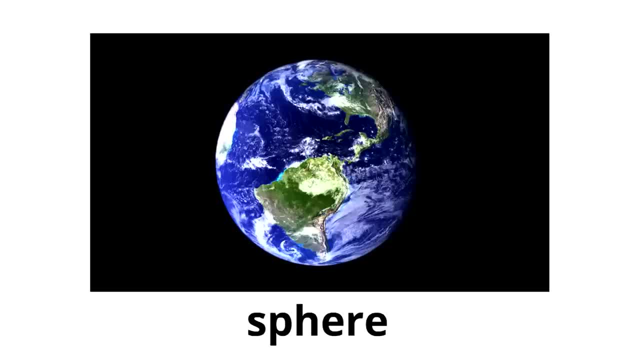 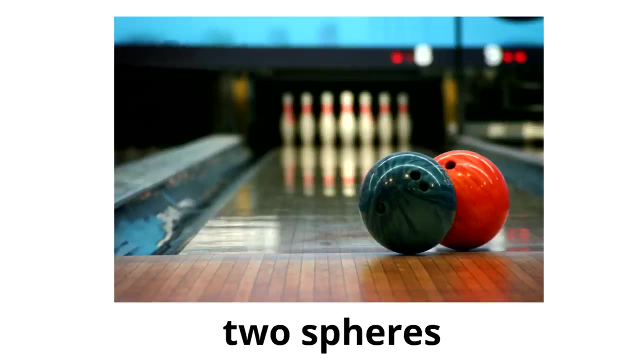 sphere. Yes, it's the earth. It's where we live. Our planet is a sphere. How cool is that? Our own planet is a sphere, Perfectly round. It's a sphere. In this picture we have two spheres. Can you spot? 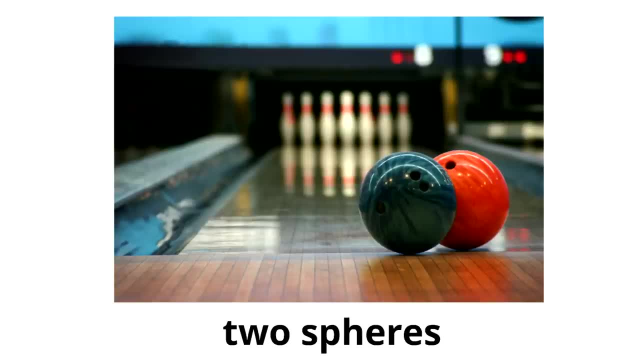 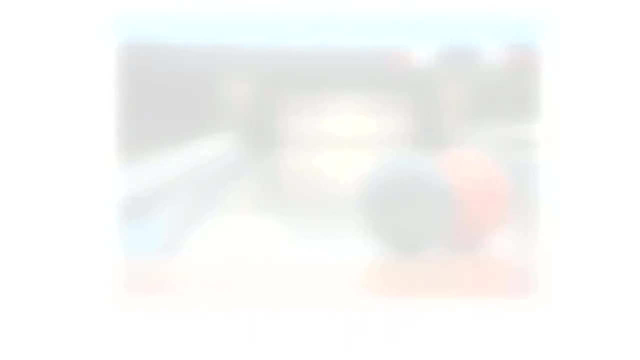 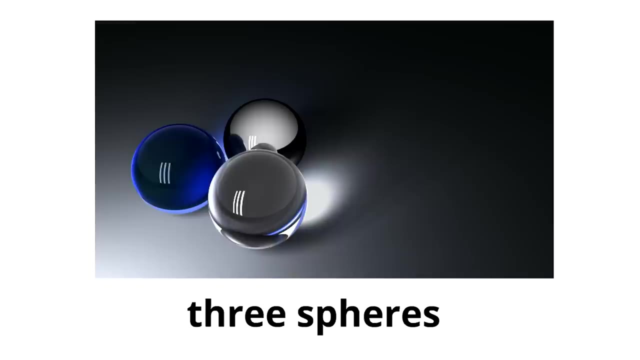 them. Yeah, the two spheres are the two balloons, Balls, Perfect, round spheres. Spheres are all around us. Here we have a group of three spheres. You can count them right now: One, two, three spheres. all together The shape of a ball, a sphere. 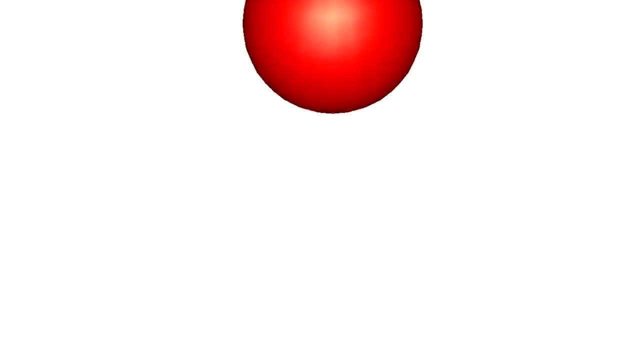 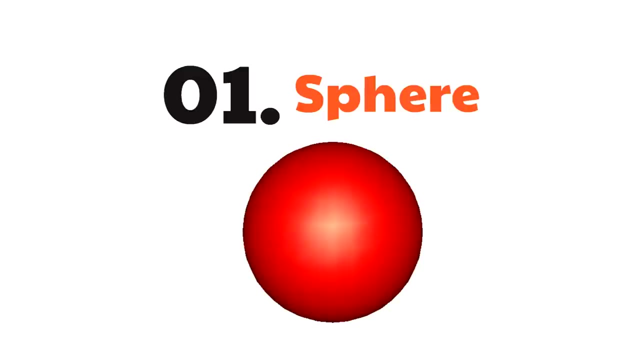 Perfectly round. Well, there you have it: The sphere. What a cool 3D shape. to start with, It's round. There are examples all around us. The sphere round us. It's just so cool. You know what The 3D shapes are going to get even better. 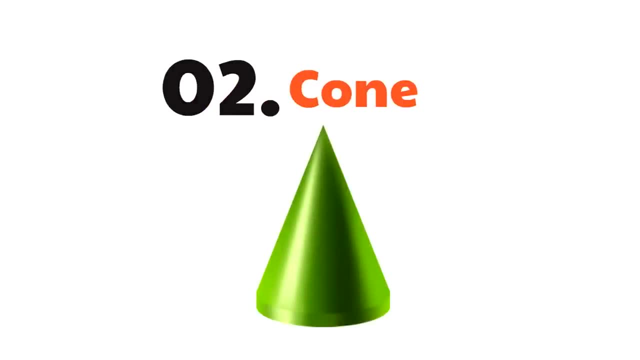 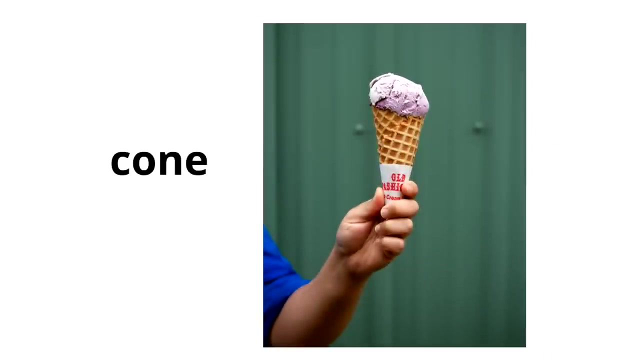 Our second 3D shape is the cone. The cone is a really cool shape with a circle as the base or the bottom. It all comes up to one point called a vertex. Here's an example of a cone. I think we all love the ice cream cone If it doesn't have any ice. 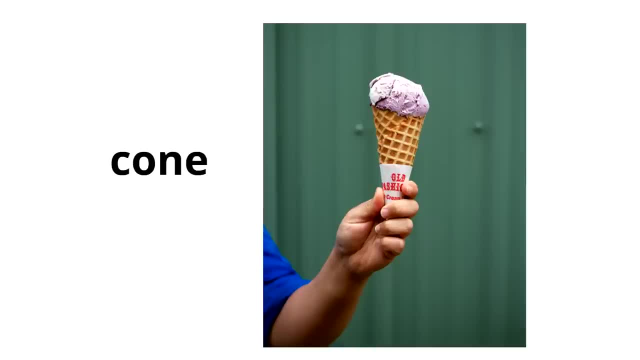 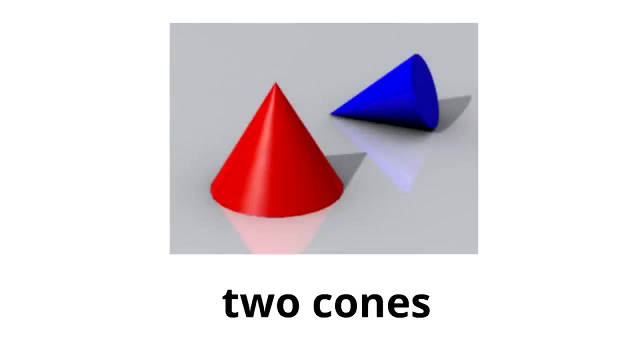 cream in it and you flipped it upside down, able to see the circle base, and it all comes up to one point called the vertex. here are two cones, a red cone and a blue cone, and you can see both cones have that circle base and all comes up to a vertex. what wonderful cones have you. 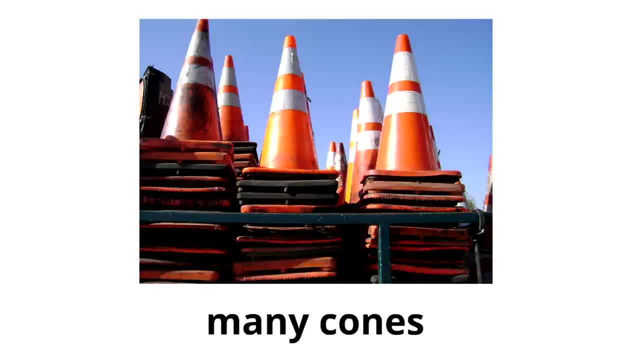 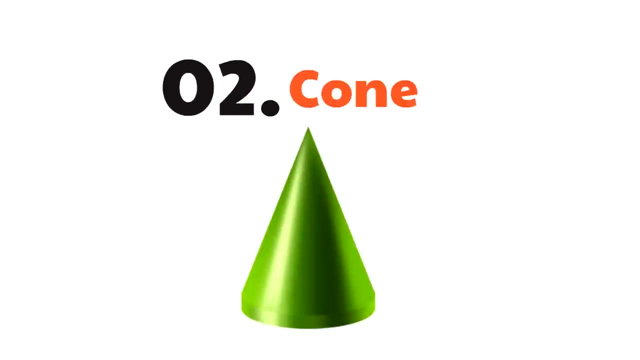 seen these before. they're traffic cones. here are many cones. I didn't count all of them, but there's a lot and they're wonderful, wonderful cones. so that's our second 3d shape: the cone, a wonderful cone, with the great circle base. it all comes up to one point called the vertex. how awesome is that? our third 3d shape. 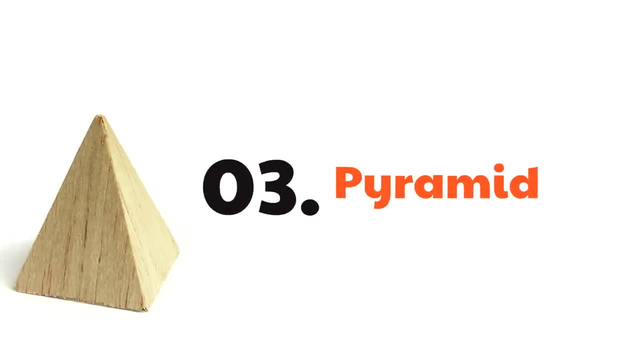 is the pyramid. I love the pyramid, the pyramids, great. it comes up to one point, just like the cone, except the base is a square, square, and the cone is a square, and the cone is a square, and the cone is a square and the sides, instead of being smooth, they are triangles. okay, like these are. 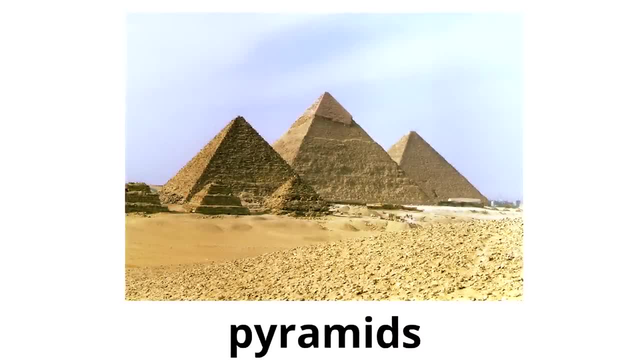 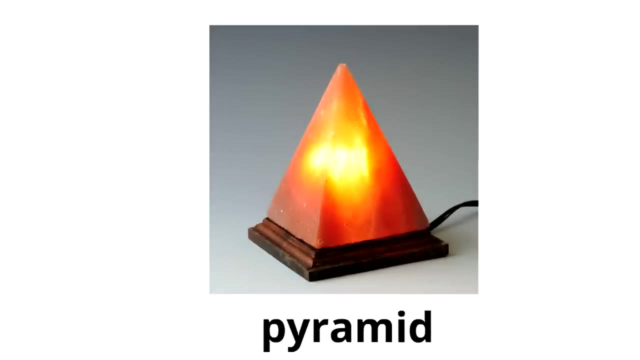 awesome. these are so cool. the pyramids of Egypt. you see that they have the triangle sides and the bottoms of these pyramids are square. they're awesome examples of the pyramid. this is a pretty cool pyramid. it's a decoration that you plug into the wall, but it's a great example of what a pyramid looks like. the 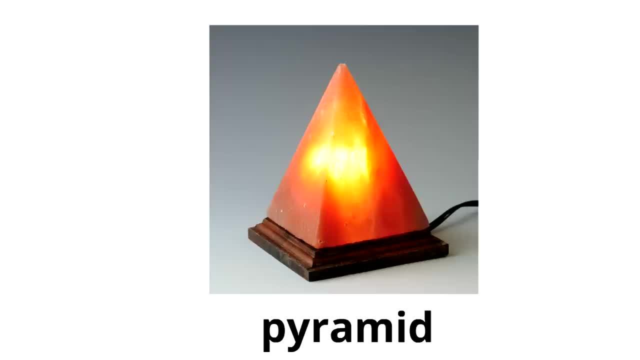 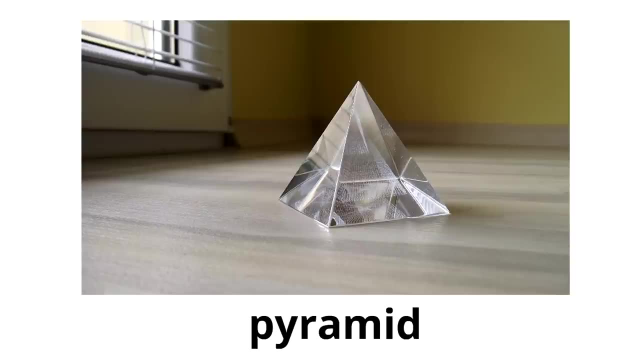 bottom, or the bottom of the pyramid looks like a pyramid. the base is square, and then there's the triangles on the sides. how cool is this? here's another pyramid. it's made of glass. there are so many decorations and things around, maybe even your house, that are shaped like a pyramid, because 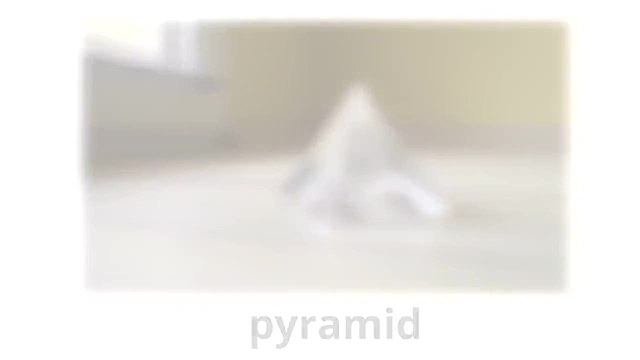 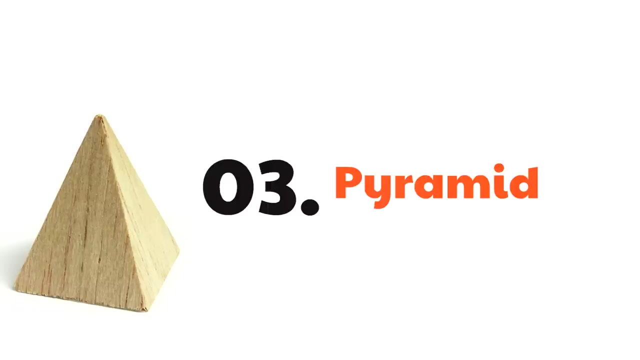 pyramids look so cool. people love putting them everywhere. there you go. I mean, you know the pyramid, it's a good shape. you know you see a lot of them around. they've got the square bottom or base, and the the triangle is always trên. WHAT LAST, WHAT IS THE BEST MRIGHT WAS THIS REVIEW. 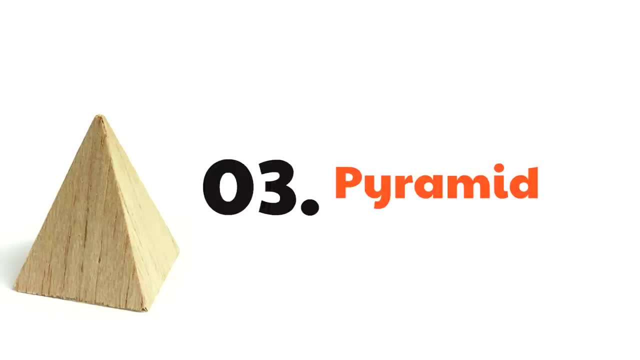 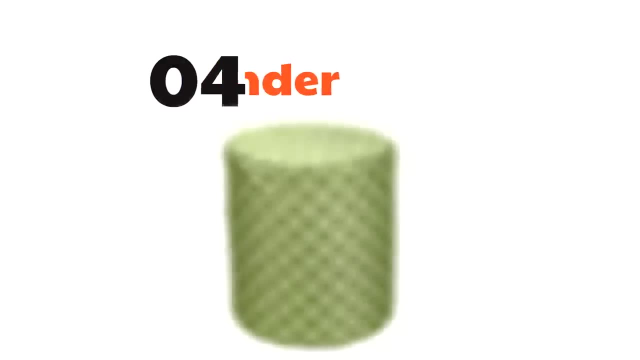 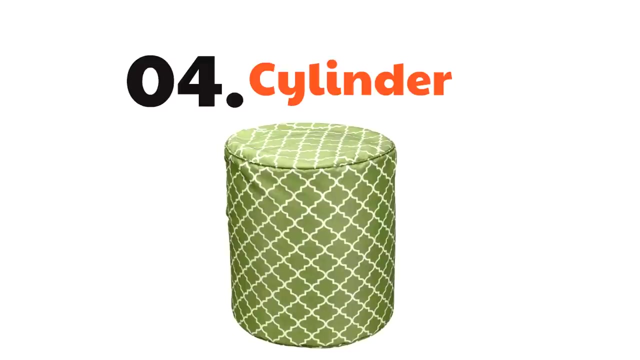 Triangles on the sides and all goes up to a vertex. It's a classic shape. It's pretty awesome. Our fourth 3D shape is the cylinder. Now, a cylinder is easy to spot because it's got a circle on the top and a circle on the bottom and it's smooth all around. 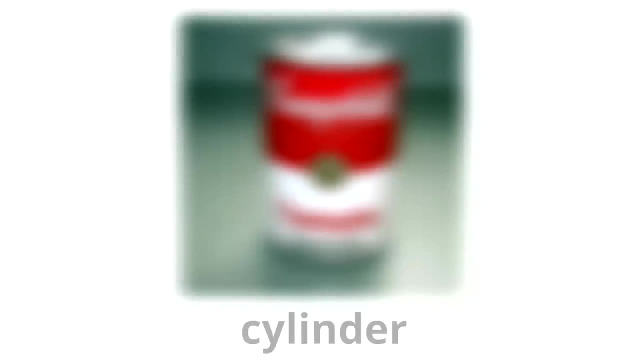 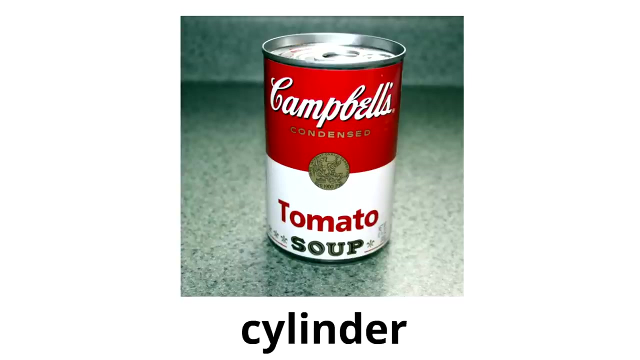 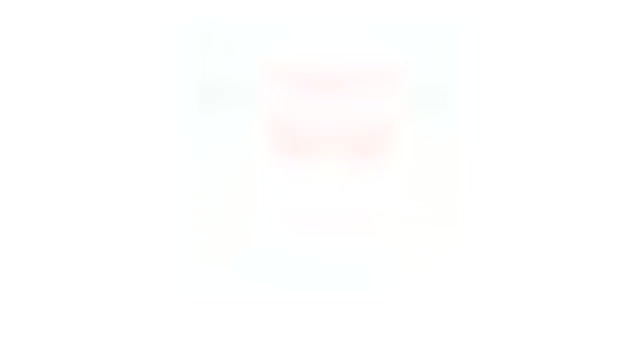 Here we have a can of soup and it's a cylinder. It has a circle on the top, a circle on the bottom and it's smooth all around. All cans and most jars are cylinders. Here we have three cylinders. They're candles And can I tell you a secret, Most candles are cylinders too, right? 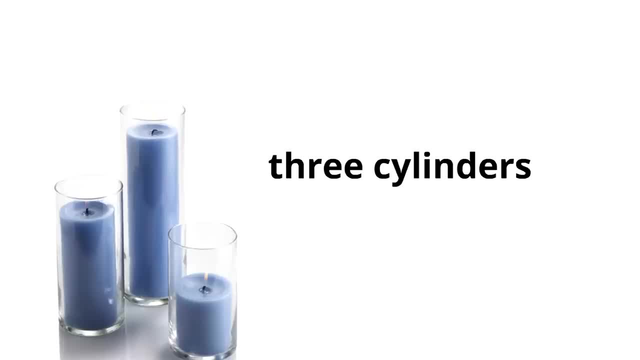 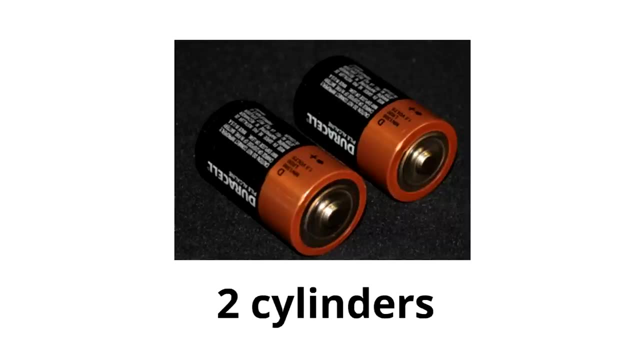 Oh, my goodness, this is just too crazy and too awesome. Here are two more cylinders. Are you kidding me? Are you kidding me? Even batteries are cylinders. Cylinders are seriously everywhere: A circle on the top, a circle on the bottom, and smooth all around. 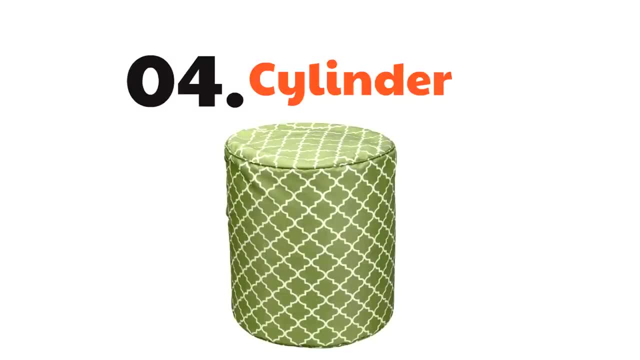 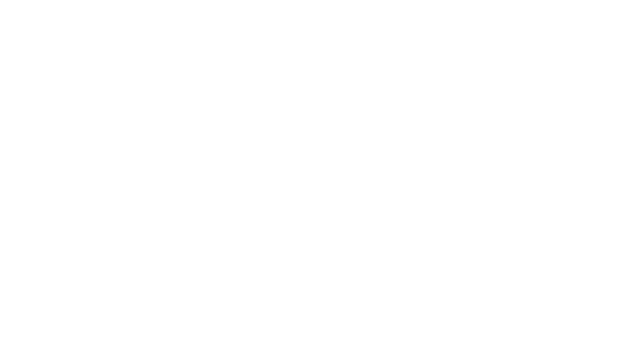 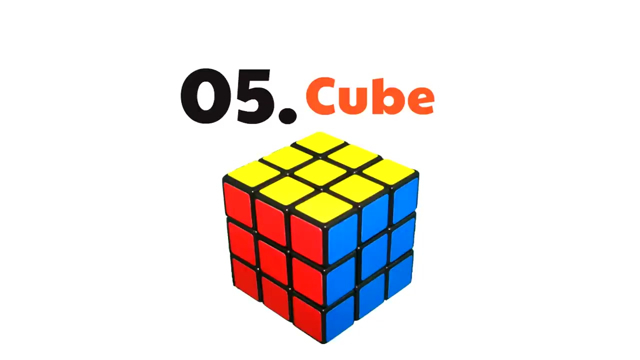 I mean, really the cylinder is everywhere. I mean you know the circle on the top, circle on the bottom, smooth, all around Cylinder, like what in the world? You have to be everywhere. okay, The next 3D shape is the cube. The cube is the 3D version of the square. It has six sides or faces that are all squares. 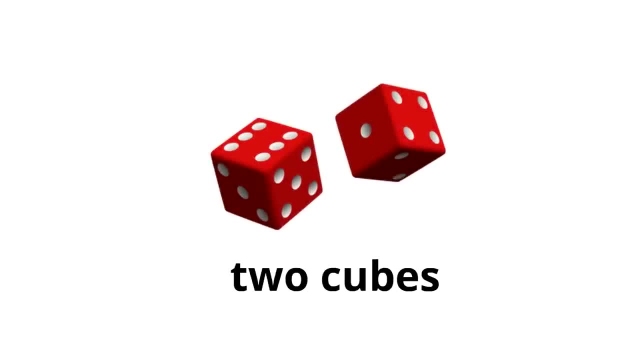 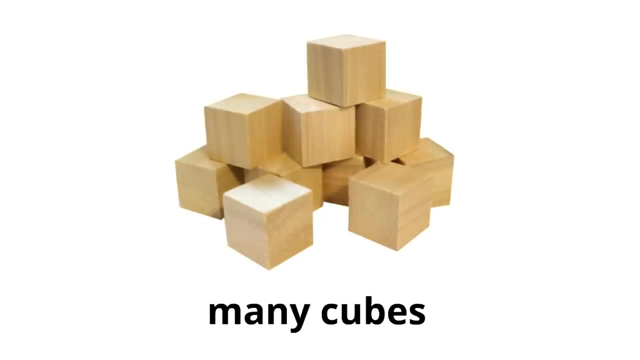 Here we have two dice. Dice are in the shape of a cube, So these two dice are two cubes. They have six sides or faces that are all squares. Here we have many cubes. These are cubes that are made out of wood. Each of them have six sides, or faces that are all squares. 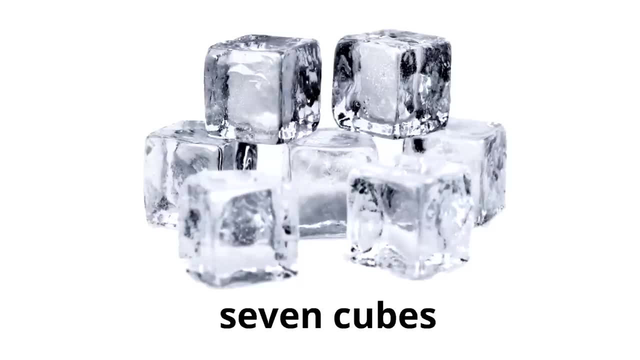 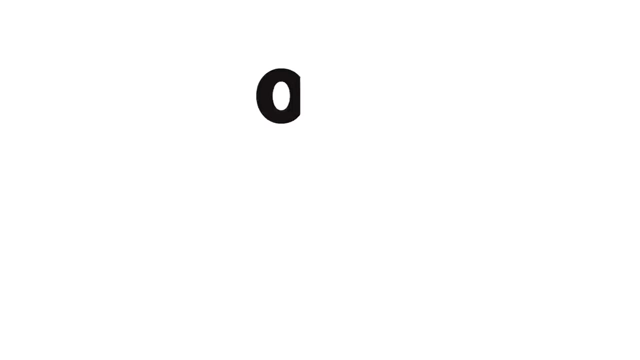 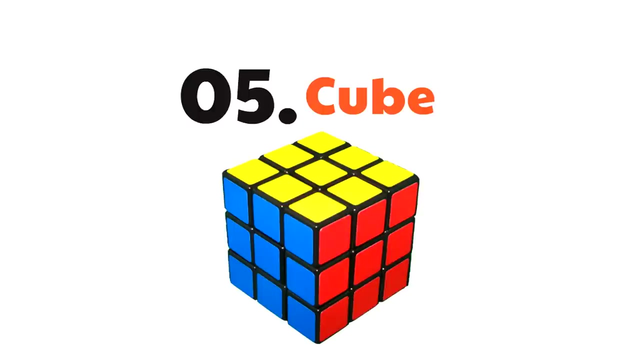 Here are seven cubes of ice. Have you ever had a warm drink and you need to put ice in it? It's awesome because it has this great shape, The shape of a cube: Six sides or faces, all squares. I mean, there you go, The cube right, The 3D version of a square, And it's got squares all along the sides right. There are six sides or faces, all squares, And I don't know. I think it's a pretty cool shape. 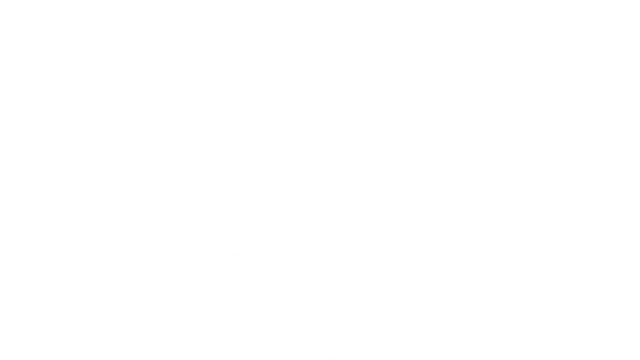 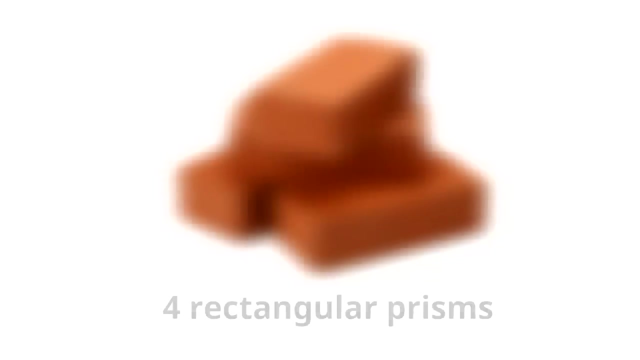 Our final 3D shape is the rectangular prism. The rectangular prism is the 3D version of the rectangle. It has six sides, or faces that are all squares, faces that are all right, okay. an awesome example of the rectangular prism are bricks, and here we have four bricks, which are four rectangular prisms. the 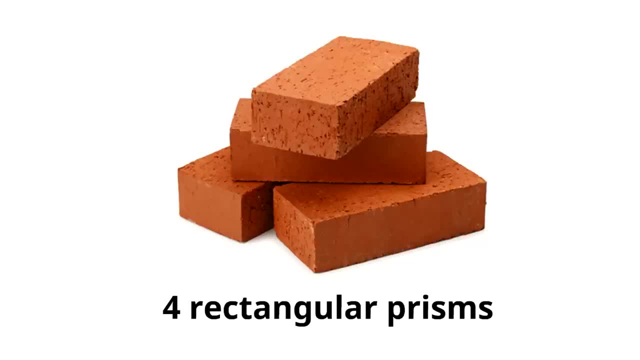 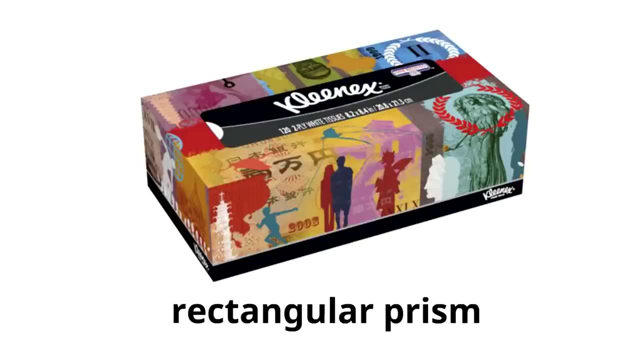 3d version of the rectangle. you may have seen this in your classroom or in your home. it's a Kleenex box, and the Kleenex box is a great example of the rectangular prism. it's got six sides or faces that are all rectangles, okay, so 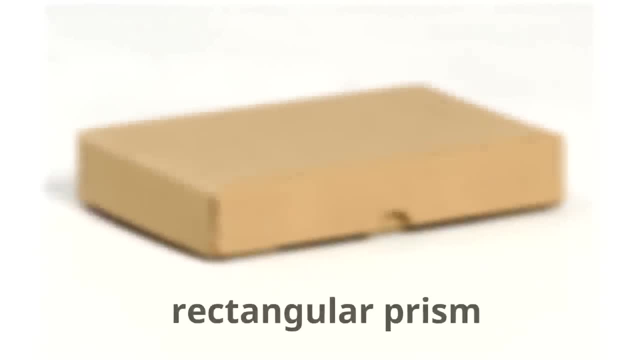 the secret is, most boxes are rectangular prisms. so here's another rectangular prism and it's a box, and it's a shorter box, but it still has rectangles all around and it's a rectangular prism. what else can we say? it's a cool shape. the rectangular prism is the 3d version of the rectangle. it has six sides, or? 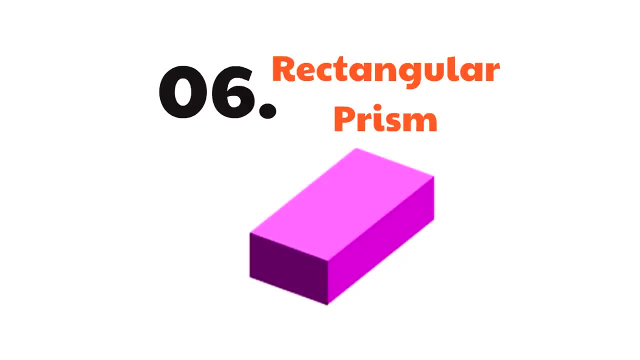 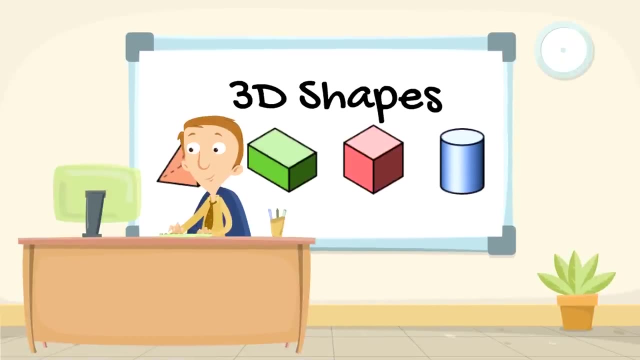 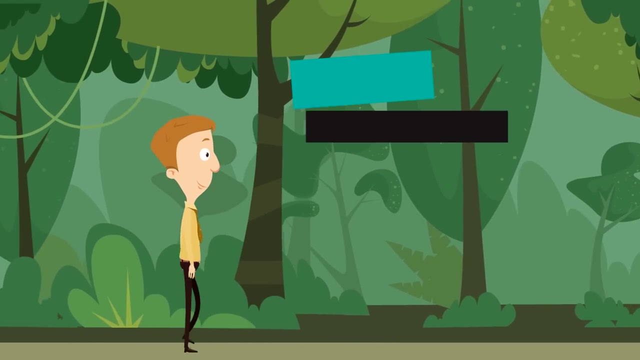 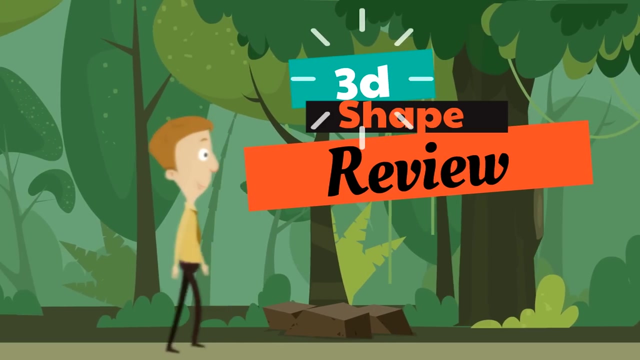 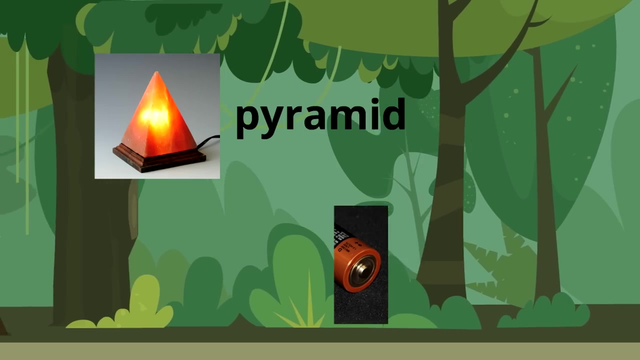 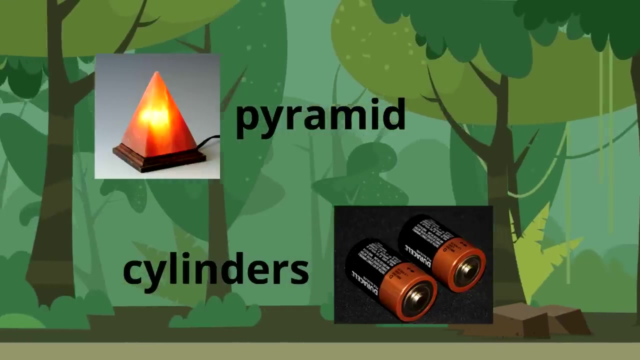 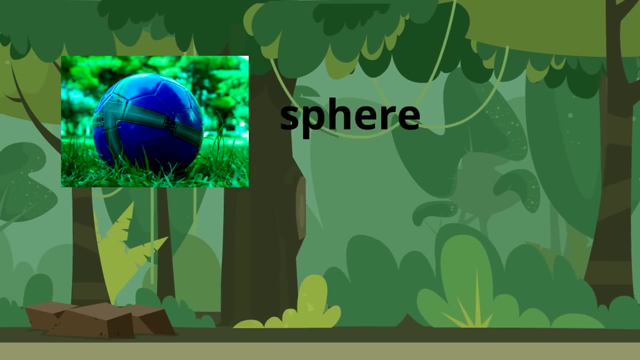 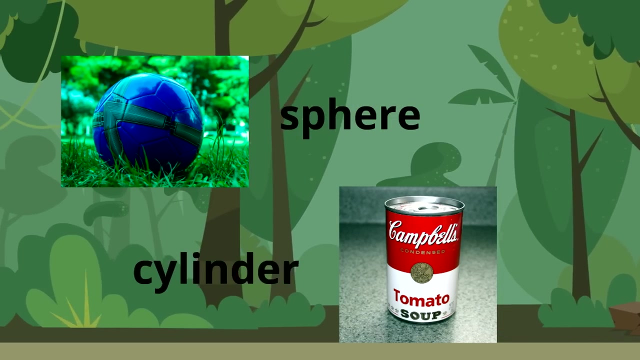 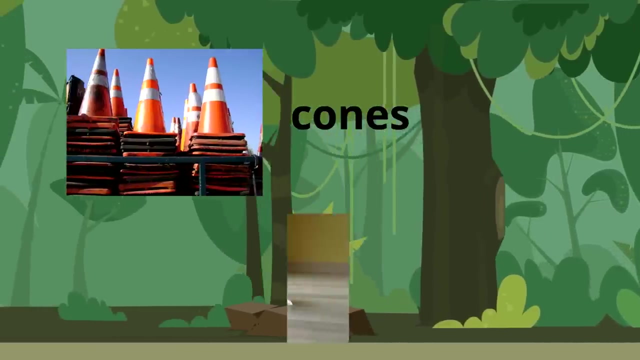 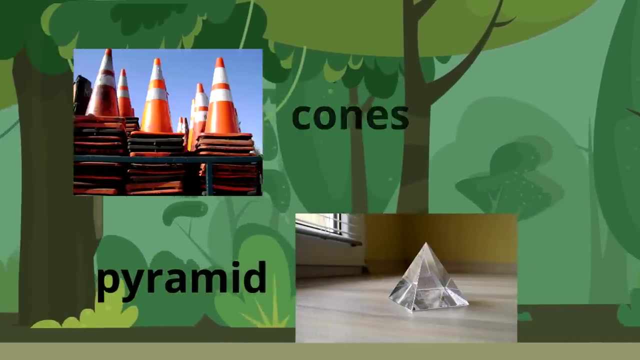 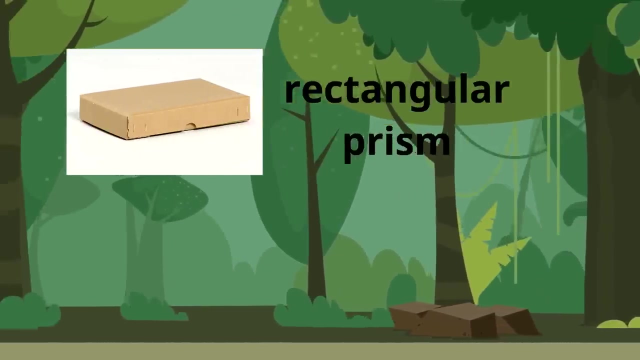 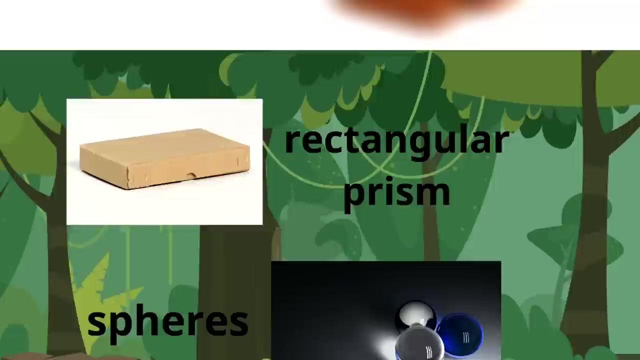 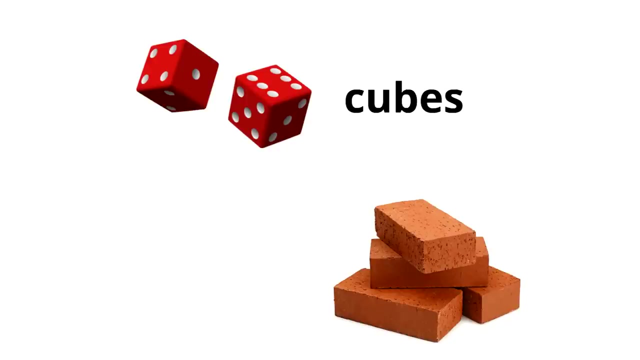 faces that are all rectangles and it's just a neat shape to have around. I think I mean you know, yes, cool, hey. so let's review pyramid cylinders, sphere cylinder cones, cylinder cylinder, cylinder cylinder, pyramid, pyramid, rectangular, prism spheres. let's do some more on the top. here we have cubes. we can tell that because it's. 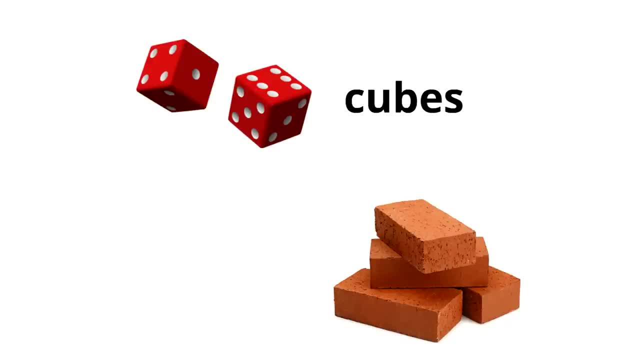 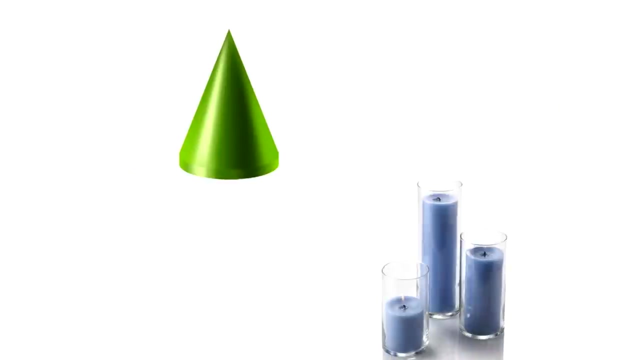 the 3d square. it has six sides or faces. each of them are squares is pretty cool. do you remember what shape these bricks are? yeah, a rectangular prism. they are rectangular prisms. they're the 3d versions of the rectangle. at the top we have a cone a. 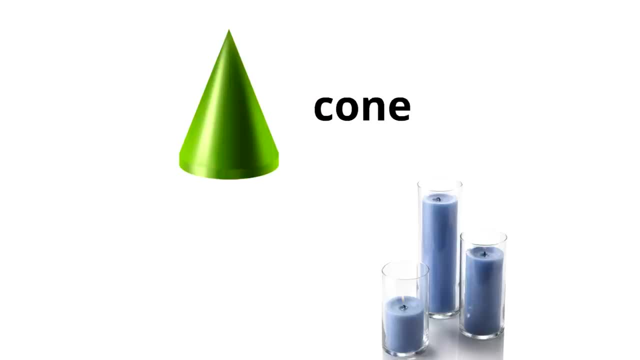 cone. it's got a circle base on the bottom and a cone on the bottom and a cone on the on the bottom and all comes up to one point called a vertex. Do you remember the shape here on the bottom? These are three cylinders. They have a circle on the top and a circle. 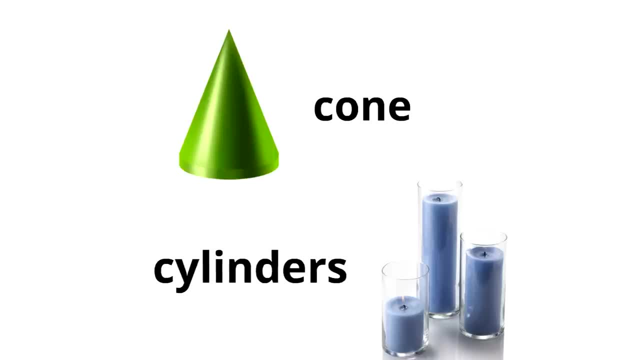 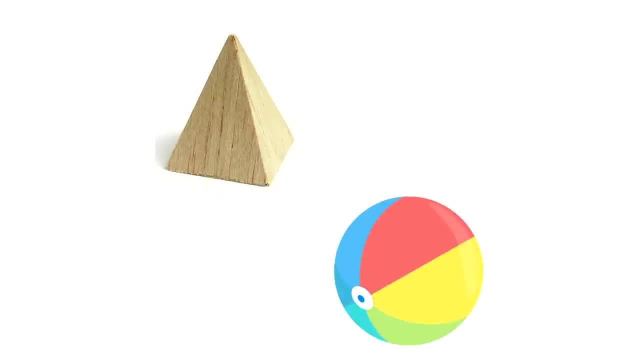 on the bottom and it's smooth all around. You're doing such an awesome job. Seriously, it's so cool. So what's this top shape? Do you remember? Yeah, it's a pyramid. A pyramid has a square base, It comes up to one vertex or one point, and it has triangles as the sides. 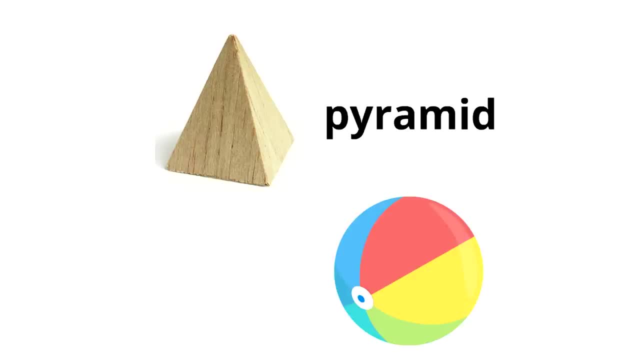 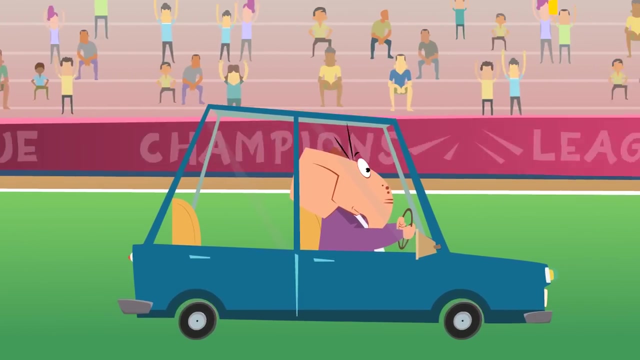 Alright, do you remember this last shape here on the bottom? Yes, it's the sphere, The sphere which is the 3D circle, and we started with it And we're ending with it, and it's so awesome, Hey, whoa. okay, first of all, elephants, don't. 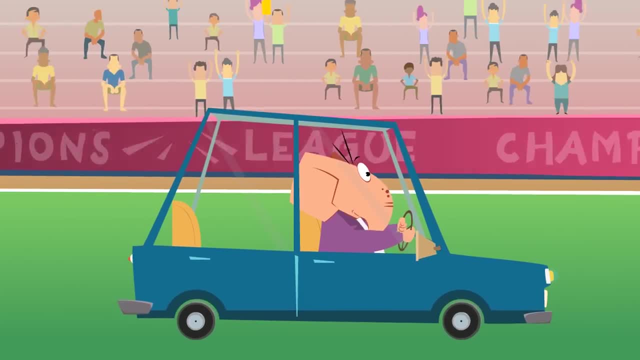 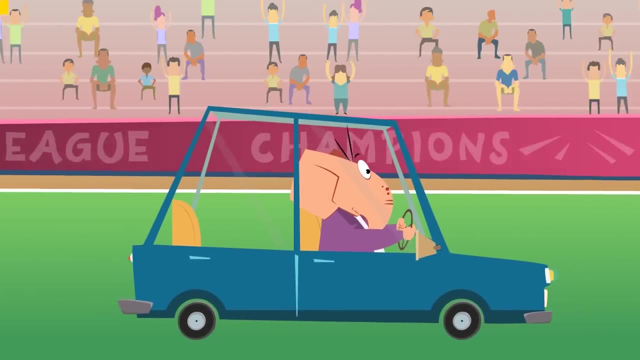 drive. Elephants can't get a driver's license and he's driving on the grass. He's driving on the grass. You're going to ruin the lawn. What's going on here? Alright, this is out of hand. Okay, elephant, I don't want to tell you what you can do and what you can't do. 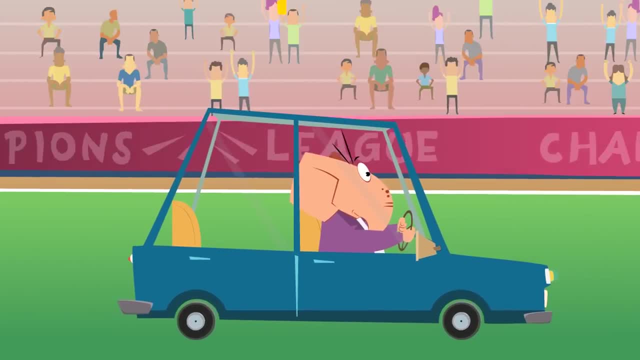 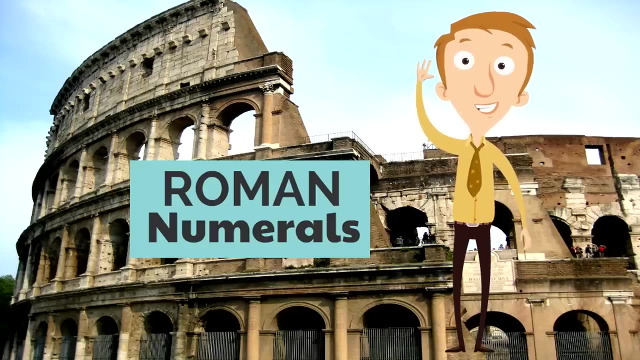 but you can't drive. Alright, Oh, my goodness. Alright. next we are going to learn about Roman numerals, which is a different way to write numbers, and it was used a long time ago in ancient Rome and it's been used since then and you can. 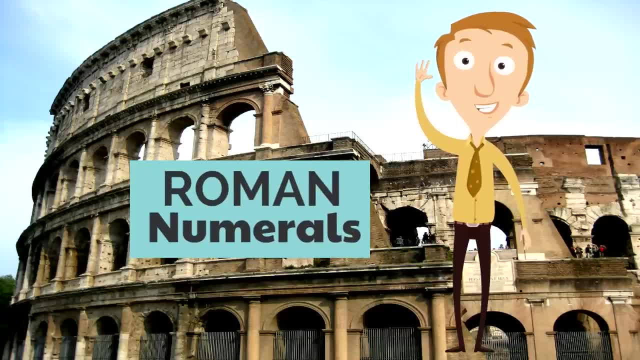 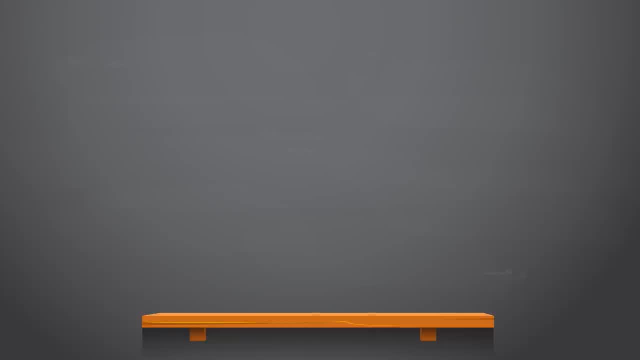 think of it almost as a secret code way of writing the numbers. It's pretty simple to learn and we're going to go through that. The first Roman numeral we're going to learn is the Roman numeral. I and I is 1.. I equals 1.. So if you see an I with a Roman numeral, it's 1.. The letter V is the Roman numeral. 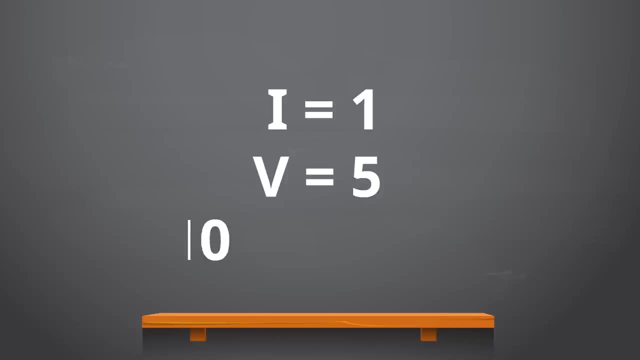 that means 5 and the letter X is the Roman numeral, that means 10.. So when you think 1, it's an I, If you think 5, it's a V and if you think 10, it's an X. 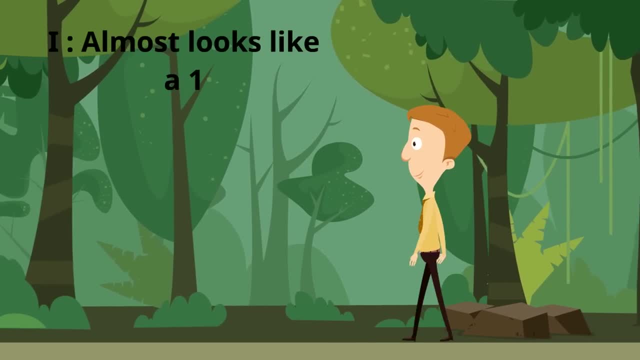 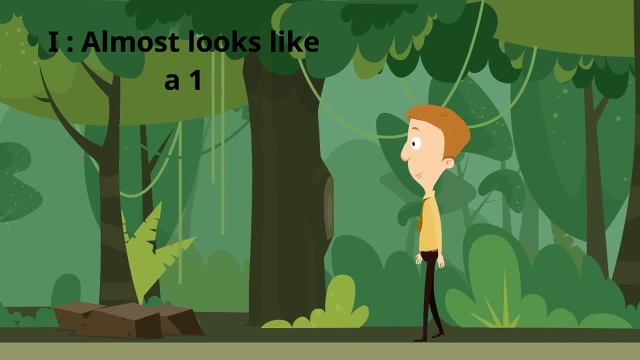 So that's it, Just those three I. it almost looks like a 1.. That's how you can remember that I is a 1.. I is the Roman numeral for 1.. A V is in the number 5 when you spell it out- The number 5,, you see that right there. 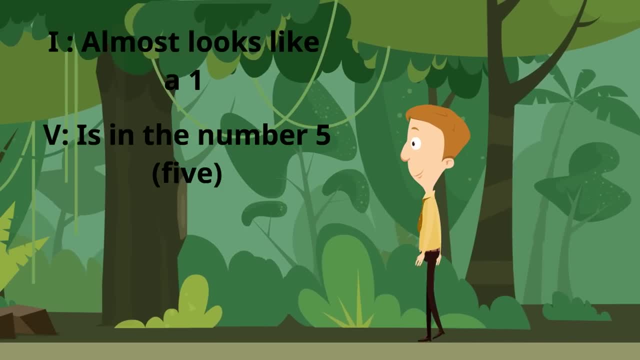 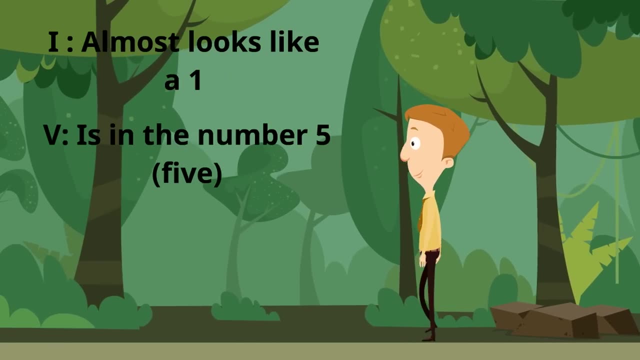 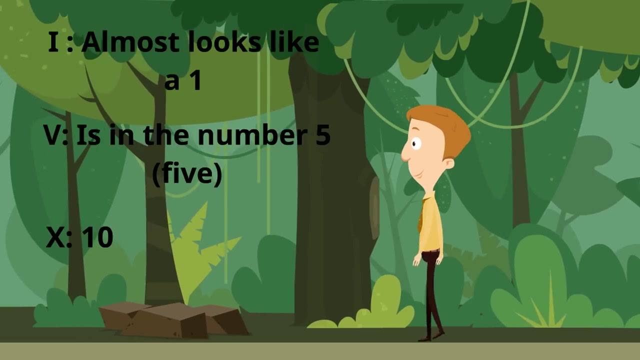 It has a V in it. So when you think of V, you know, oh, you know what. There's a V in the spelled out number 5.. So V has to be 5. Now 10 is X, and we can't think of anything that could remind us of that. So there is no memorization thing. 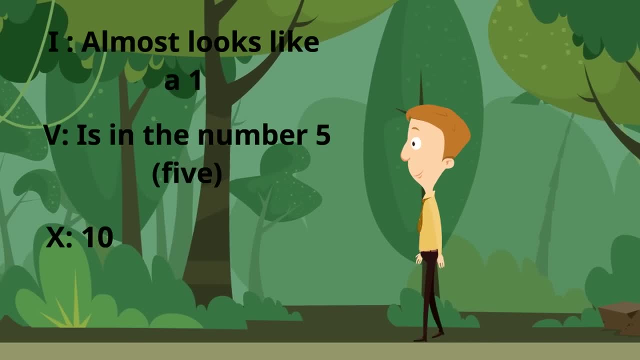 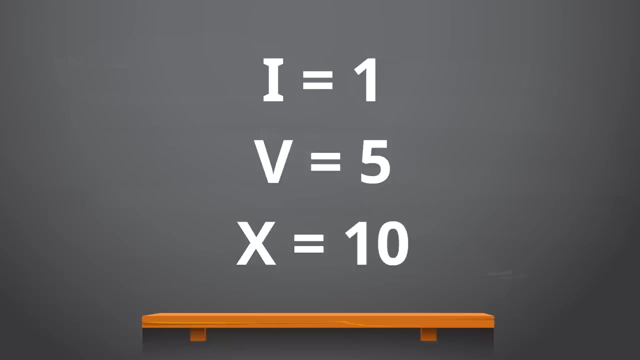 Just when you see the X, it's 10, and that's just what we're going to have to do. Okay, one last time here. I just want to make sure you get it. There's only three. I is the Roman numeral for 1.. V is the Roman numeral for 5 and X is the Roman numeral for 10.. 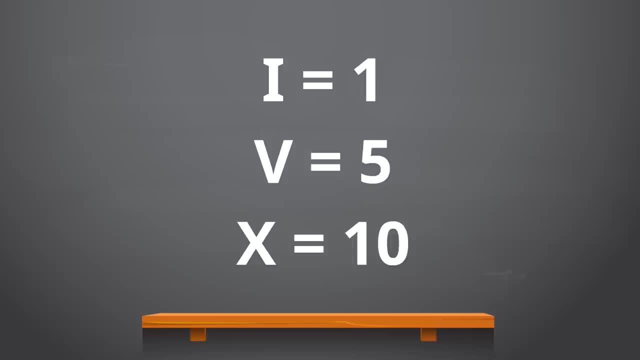 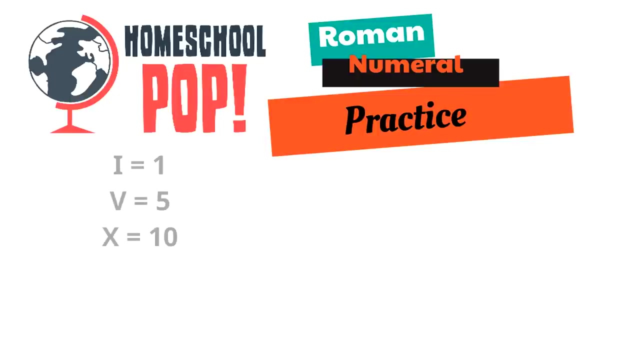 And you've got to understand that so that we can learn it And start playing kind of a game of putting them together and making numbers other than just 1,, 5, and 10.. So let's get started, So let's practice putting these Roman numerals together. 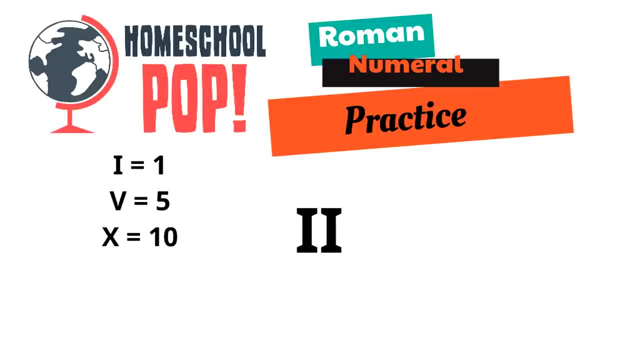 What number do you think this is? You see two I's and I is 1.. So the answer is 2.. Two I's is the number 2.. What about this one? What number do you think this is? There are three I's. 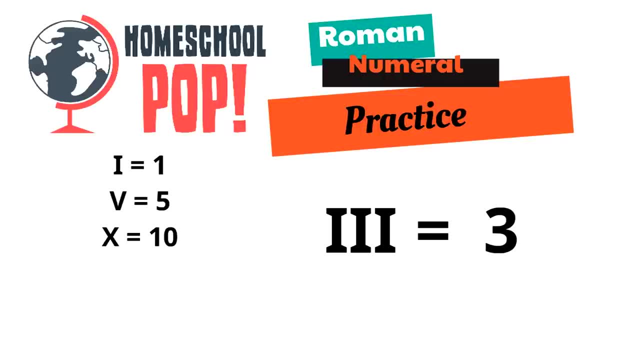 Yeah, it's the number 3.. Let's try this one. What number do you think this is? We see two X's, and X equals 10.. So 10 plus 10 equals 20.. Great job, This is the number 20.. 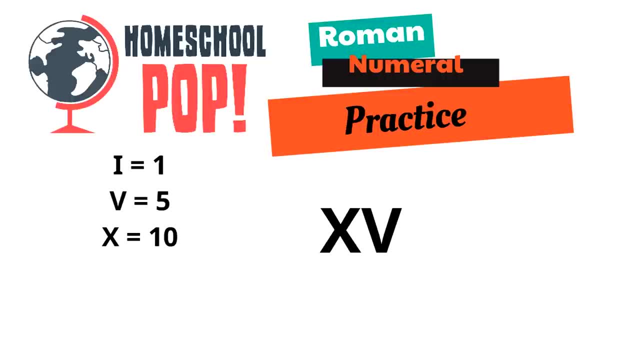 Whoa, this one is so cool. Okay, An X and a V. What number do you think this is? The X is a 10.. The V is what number? 5.. Awesome, So what is 10 plus 5?? 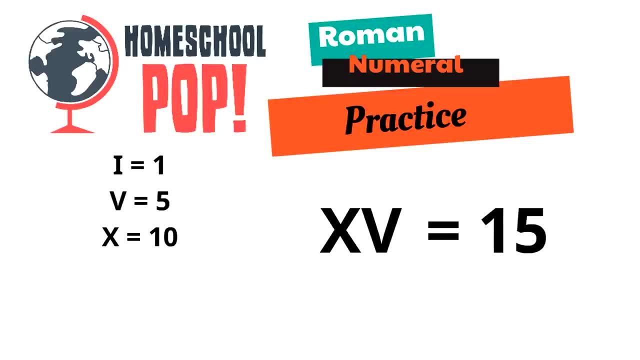 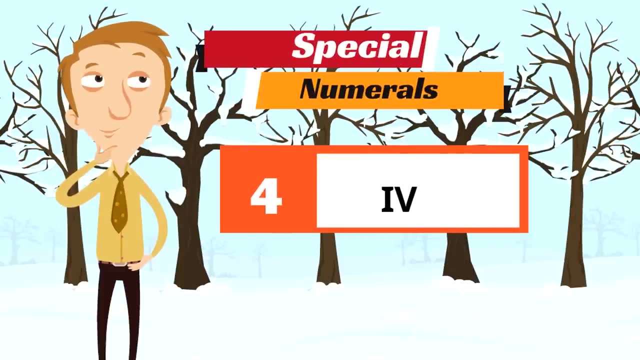 15. Whoa, thanks so much for helping out. Now that we've looked at how to put some of these together, I want to tell you about two special numerals that are a little bit different, And so you're going to have to just remember these on their own. 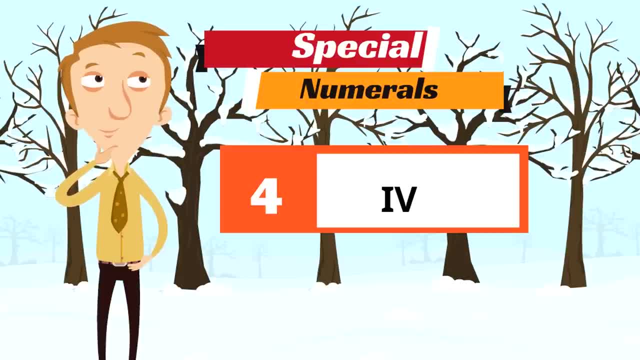 The first is the number 4.. And the number 4 is represented with an I and a V, And the I is before the V, because 4 is 1 less than 5, which is V. So remember, with 4, it's IV. 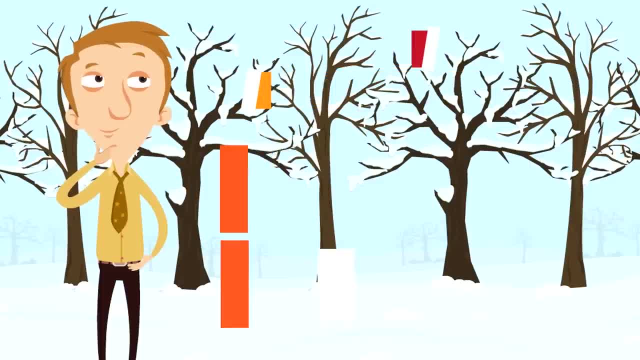 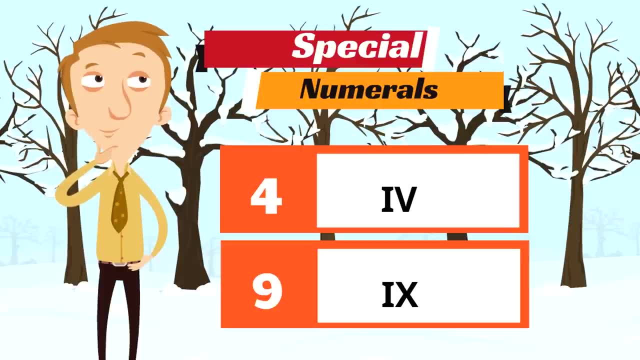 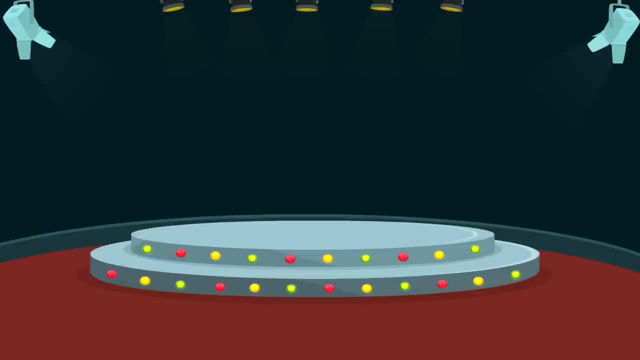 With 9, it's similar, except with the X. 9 is IX, X is 10.. And I is just before it, So 9 is IX. Okay, that was really cool. Thanks for hanging out and learning those with me. 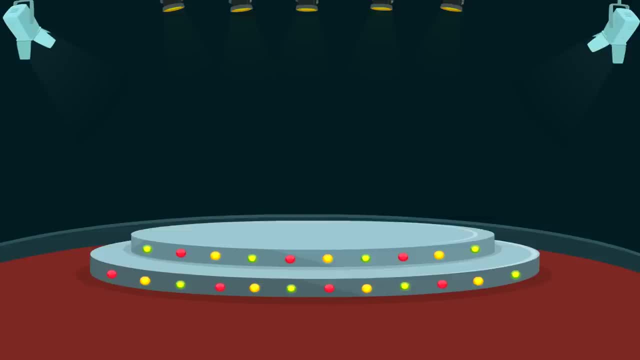 But we're not done. We want to go through all the numbers up to 30 just using the numerals And I want to see how much you've really learned. So if you'll do me a favor, as the numerals go up, 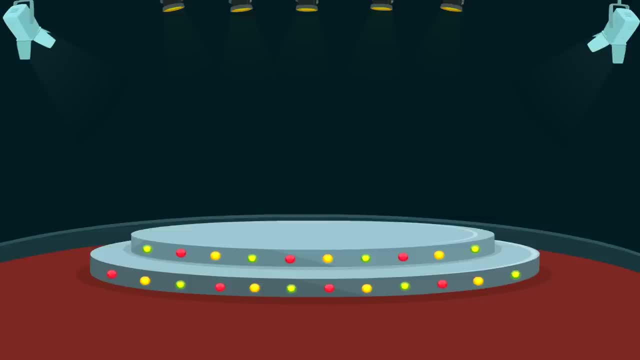 I want you to say the numbers along with me and we can practice together. Sound good? All right, let's get started. 1, 2, 3, 4, 5, 6, 7, 8, 9, 10, 11, 12. 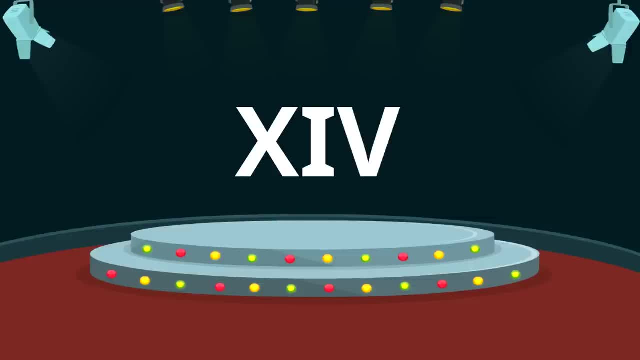 13, 14, 15, 16, 17, 18, 19, 20, 21, 22, 23, 24, 25, 26, 27, 28, 27, 28, 29, 29, 30. Well, there you have it, A new way to write numbers. 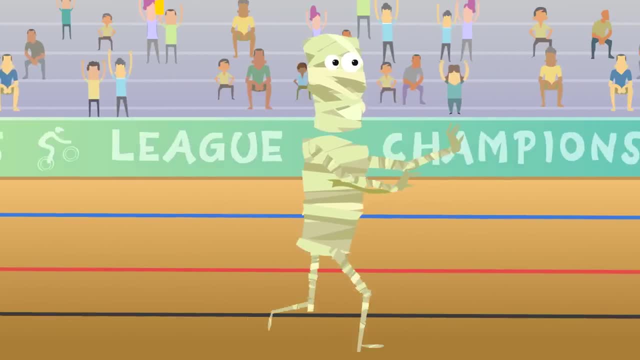 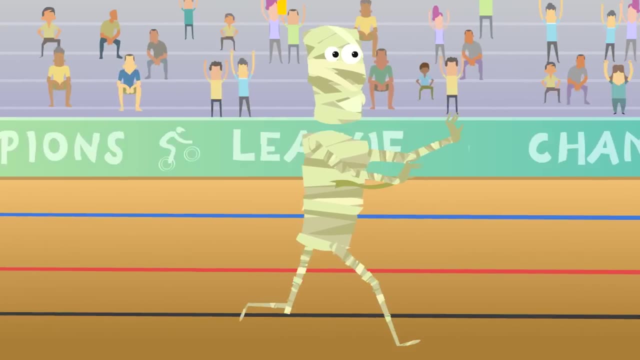 Wow, Mom, you're doing such a great job in your race. I had no idea you were an athlete. okay, I mean, with all that cloth wrapped around you, you're doing great. You're doing a great job, Just like these kids are doing a great job learning. 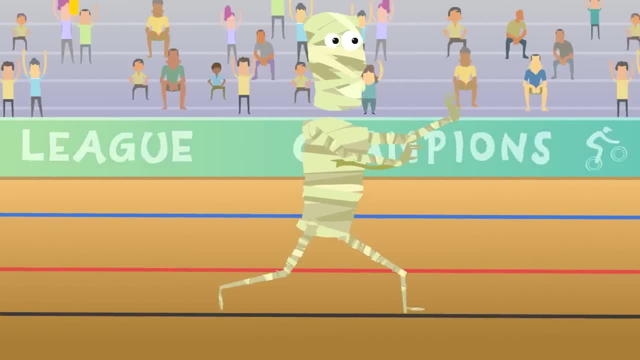 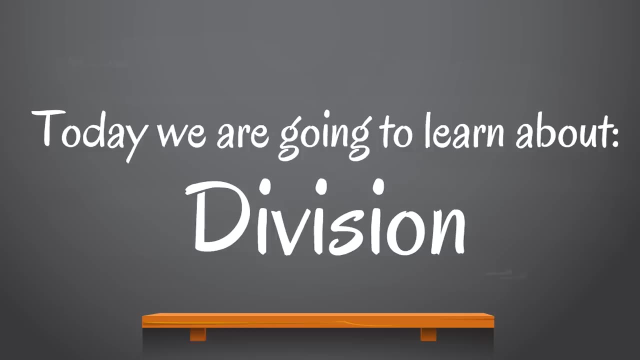 In fact, how about this? The next thing we're going to learn about is division. Division is such an awesome thing to be able to do, And you're going to have it all figured out. You're going to learn how to divide in this video. 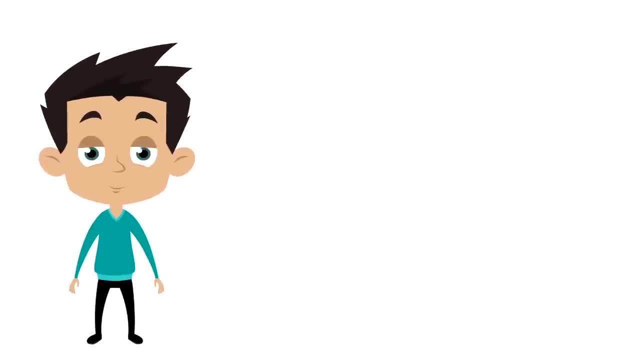 And we're going to start off with a story. There's this kid named Ethan, And Ethan loves carrots. He loves carrots so much He loves to snack on them. He loves when he gets to eat them. They're crunchy, They're tasty. 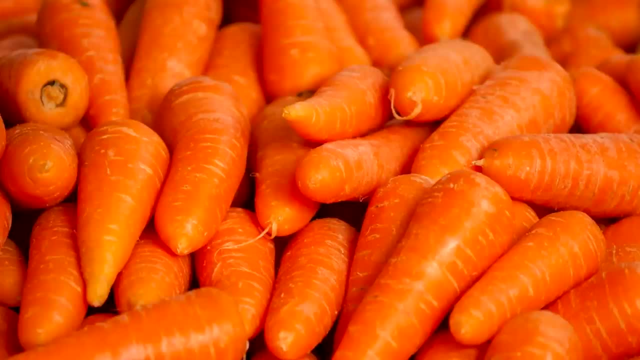 Yeah, carrots are awesome. In fact, I'm literally eating a carrot right now as I'm speaking. Carrots are great for your skin. Carrots are great for your eyes. They're amazing. They're a great snack And Ethan loves them. 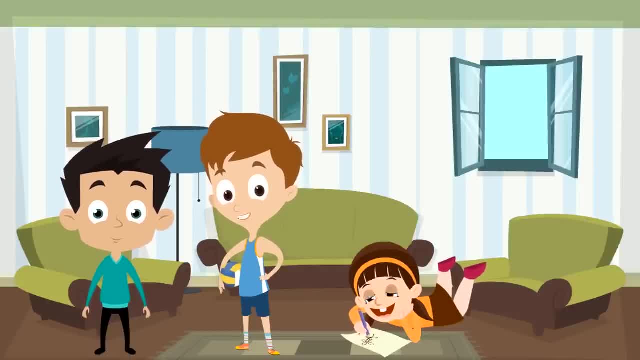 Well, Ethan has two friends over, Kevin and Chloe, And they start to get hungry. Of course, they all love carrots, Because carrots are like the perfect snack. Now, in Ethan's house, there are only three carrots. There are just three carrots. 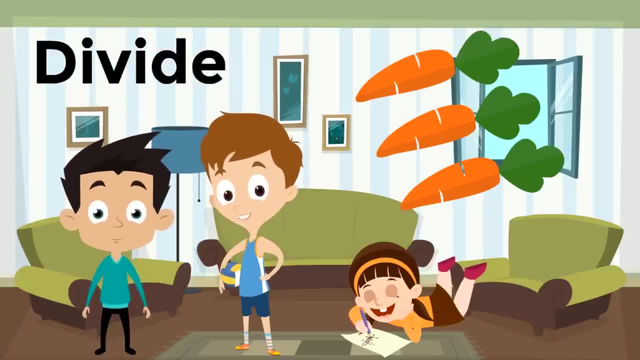 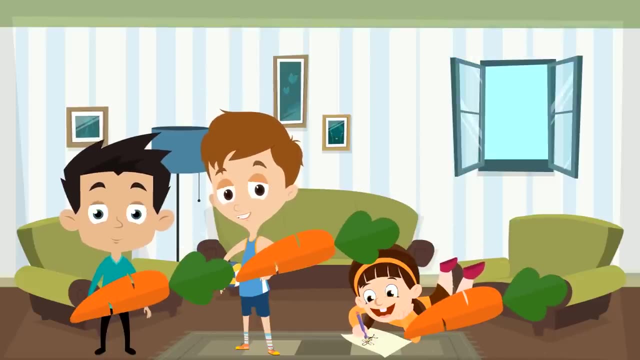 We are going to have to divide the three carrots amongst the three kids. So let's figure this out. How many carrots does each kid get, Do you know? Uh-huh, Each kid gets one carrot. Pretty simple, right? Three carrots, three kids. 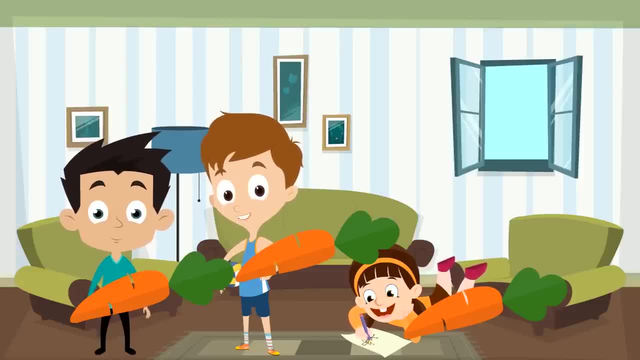 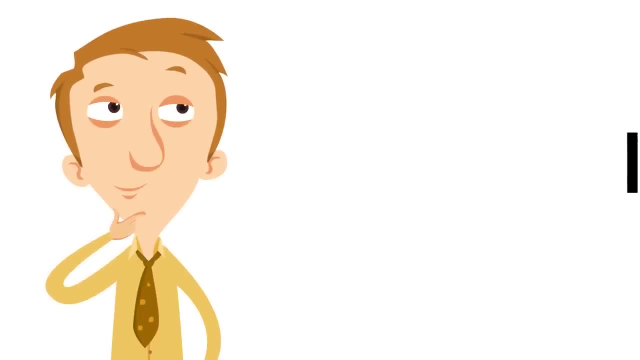 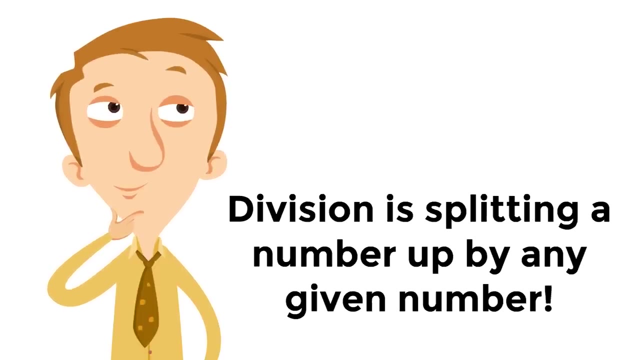 Each kid gets one carrot. Hey, did you know? we just did division. Uh-huh, We just did division. Division is pretty simple. You see, division is splitting a number up by any given number. That's it just splitting a number up. 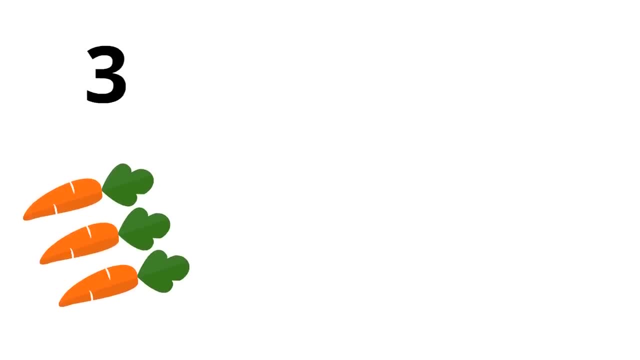 Let's look at our story again. There were three carrots and we divided those three carrots by three, There are three people, right, the three kids that love carrots, and the answer of how many carrots each kid gets is one. Three divided by three equals one. 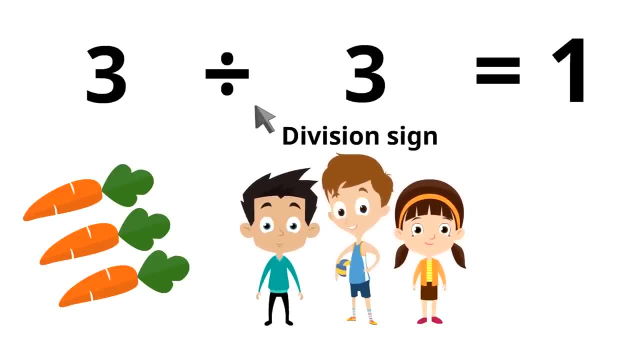 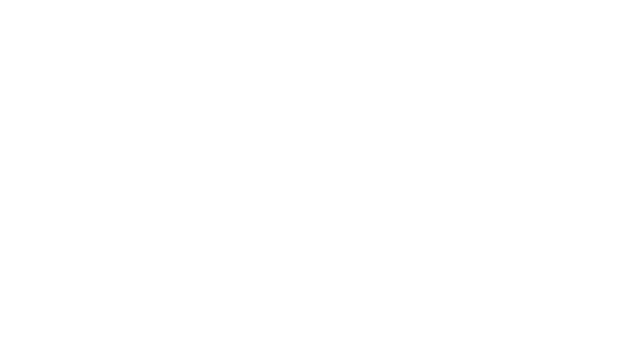 Notice. right here is the division sign. This is what it looks like When you see that sign. you could just say divided by. So this reads: three divided by three equals one. Let's try another example of division. Let's say there are eight presents, eight presents and there are four women, and we want. 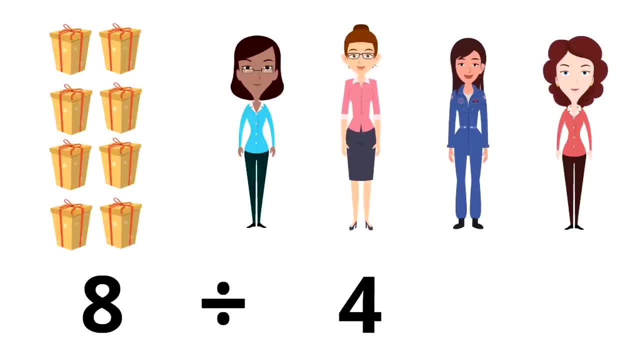 each of the women to get the same amount of presents as the other women. because we want it to be fair. Notice the division sign. We are going to divide or split up eight by four. Remember to divide is to split up. Let's split these presents up into four equal groups. 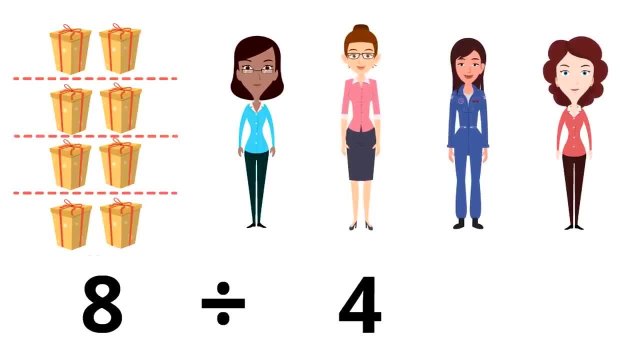 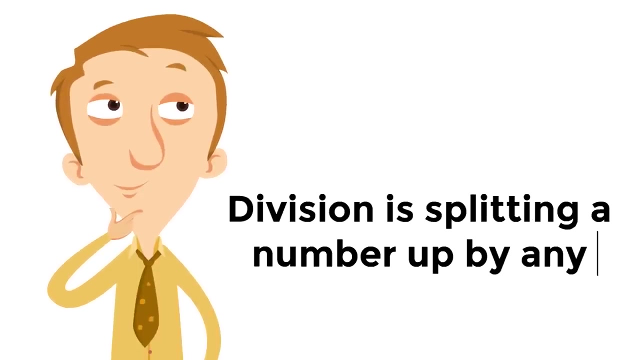 One, two, three, four. Alright, how many presents does each woman get? Uh-huh, two. Each woman gets two presents. Isn't that cool? Division is so much fun and it's so easy. Let's see, Remember, division is splitting a number up by any given number. 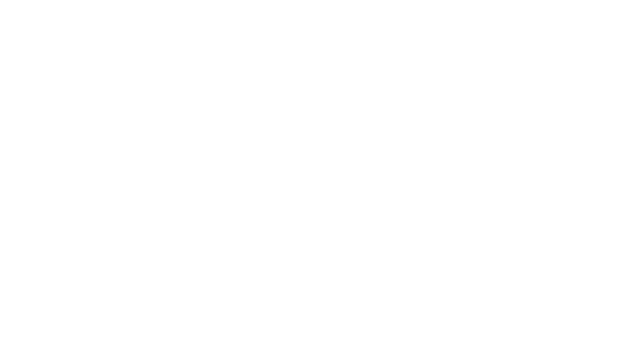 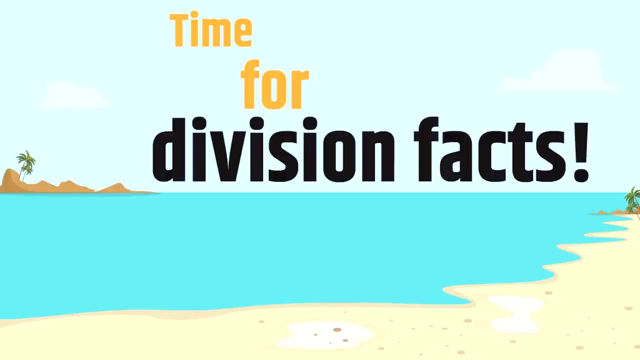 That's it, Alright. now it's time for division facts. We're going to learn some pretty interesting facts about division and you're going to be like what- Oh my goodness, Like secrets. This is super cool, okay, So just look around, alright. 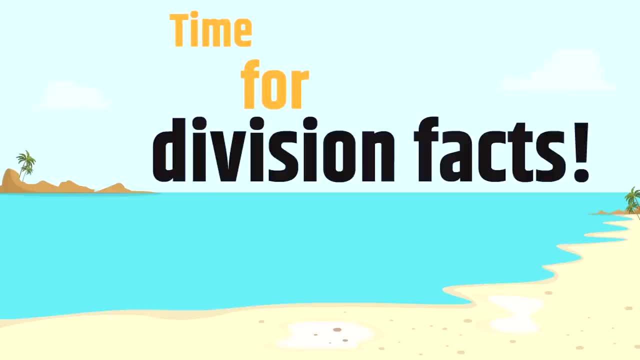 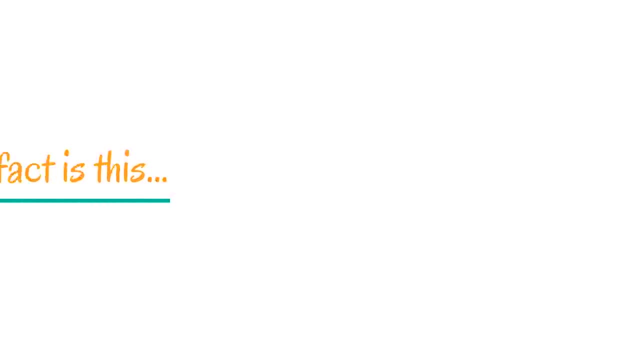 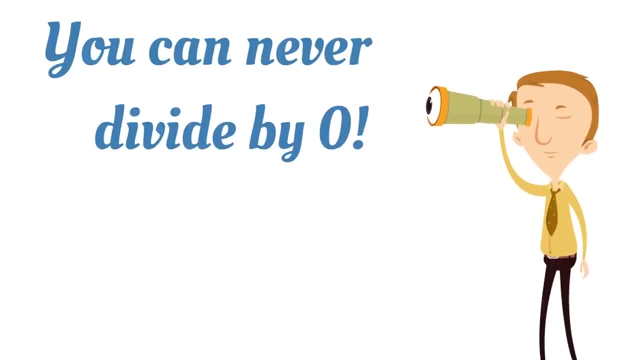 Make sure. Alright, It's time for division facts. The first fact is this: You can never divide by zero. It's true. You can never divide by zero, even if you're a rule breaker and you're like I'm going to do whatever I want. 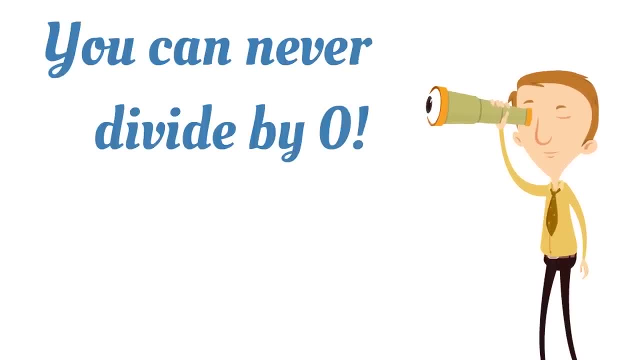 You still can never divide by zero. In fact, if a teacher ever gives you a test and you see a problem where you have to divide a number by zero, Just write on the test: undefined, because that's exactly what that answer would be. 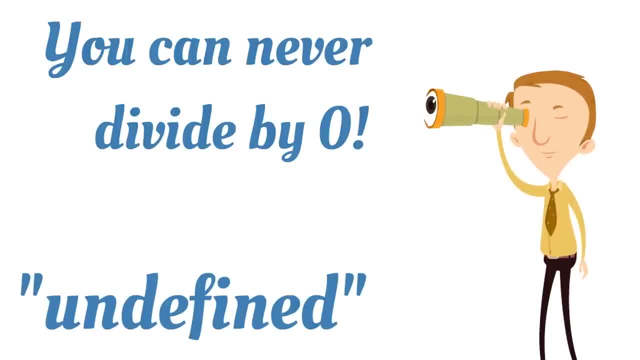 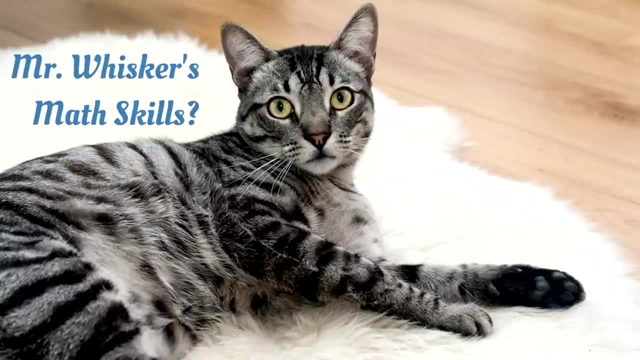 Undefined, It's impossible. Kind of like Mr Whiskers math skills. Does Mr Whiskers do math in his head all day long? Who knows? His math skills are undefined, We just don't know. It's impossible to know. 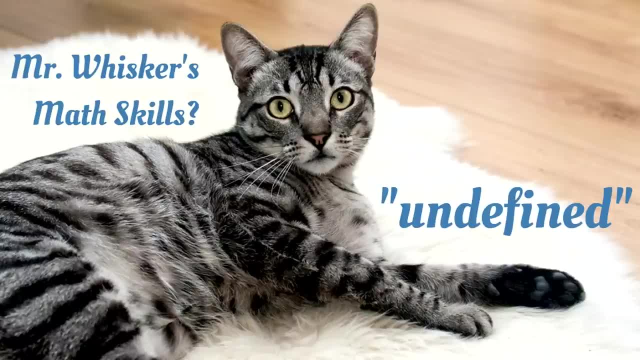 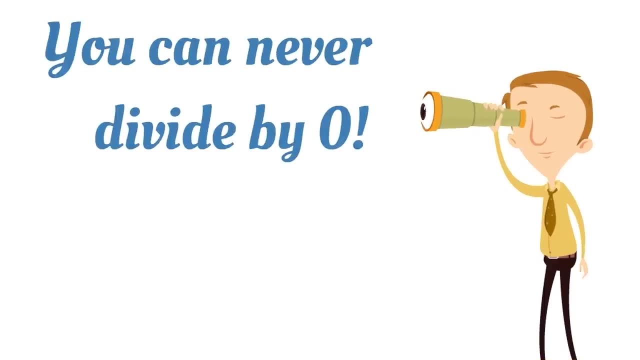 You know, Mr Whiskers might know how to do division, Who knows? Undefined. You can't divide by zero. You can never divide by zero. If you ever see any division problem dividing by zero, just write: undefined, It's impossible. 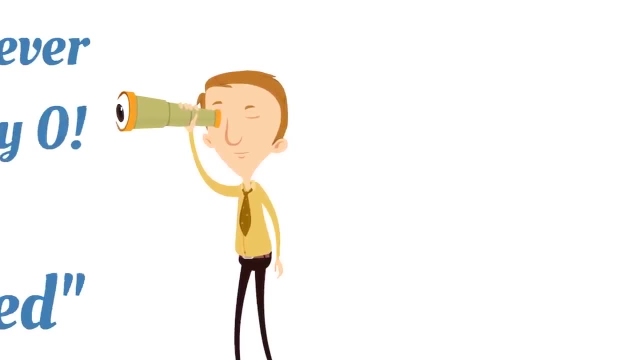 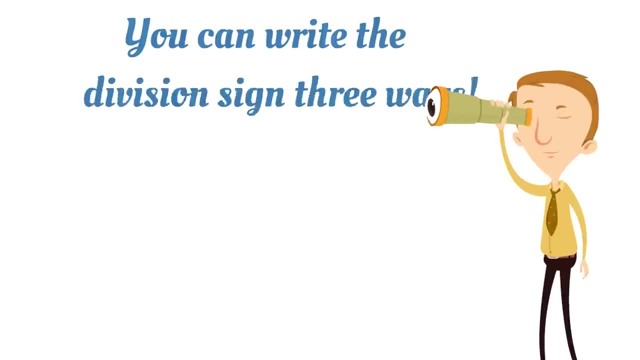 It's impossible, So just write undefined. The second fact is this: You can write the division sign three ways. Uh-huh, You can write it like the division sign, or you can write a division problem with the slash or with a horizontal line. 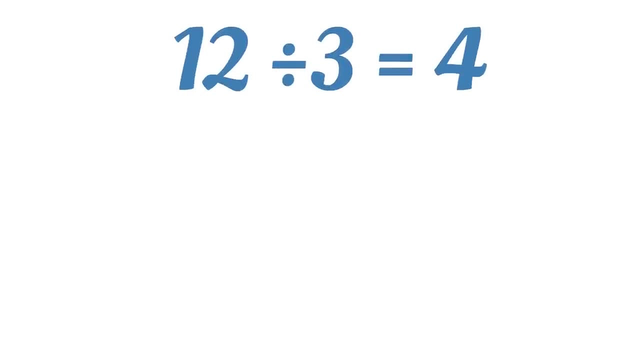 For example. look at this: Twelve divided by three equals four. That's the original division sign, the one that you might see more regularly: Undefined, Undefined, Undefined. It's the same equation written in a different way. Twelve divided by three equals four. 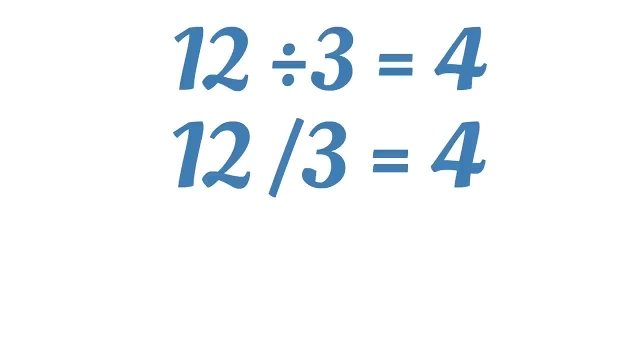 It's still a division sign, but it's a slash. It means the same thing as the original division sign. Remember, the division sign can also be a horizontal line. Twelve divided by three equals four. That looks like a fraction, doesn't it? 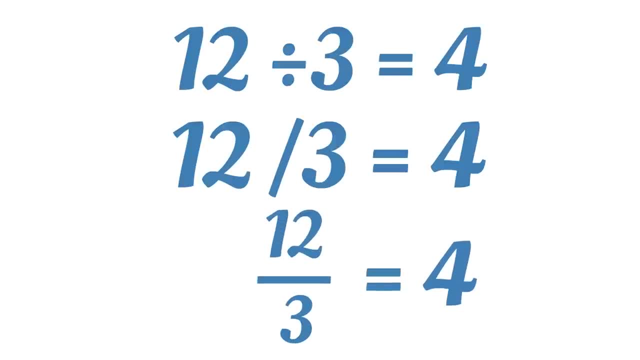 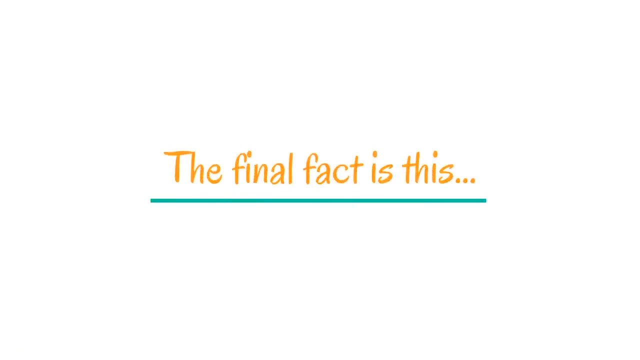 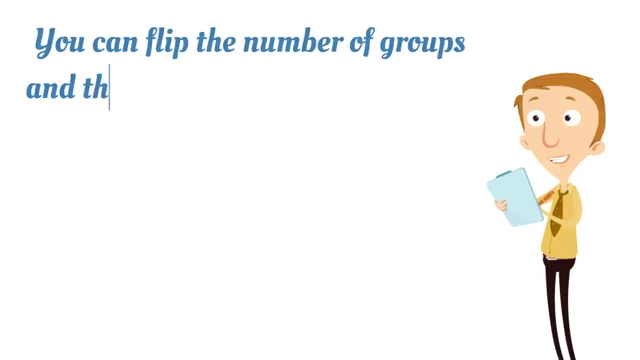